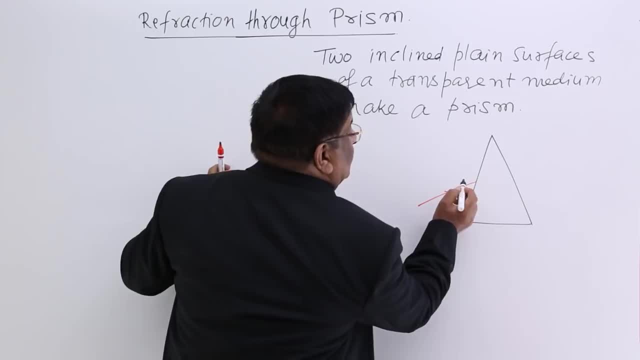 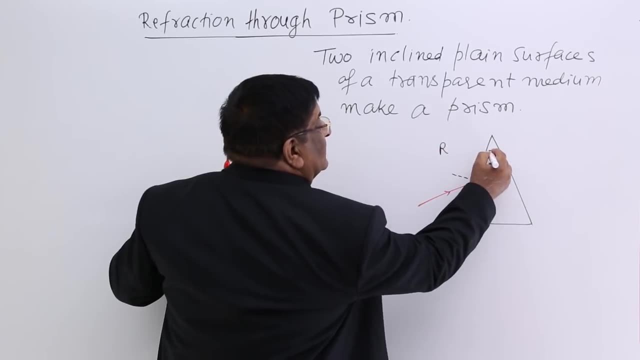 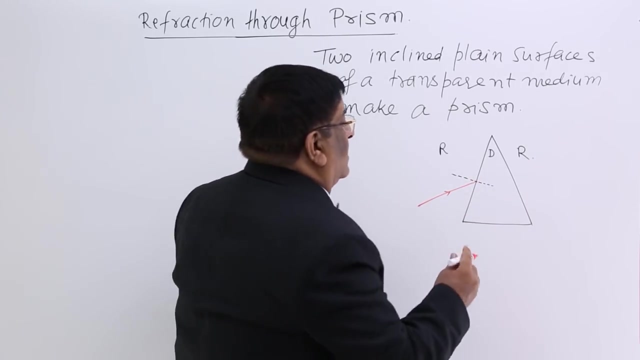 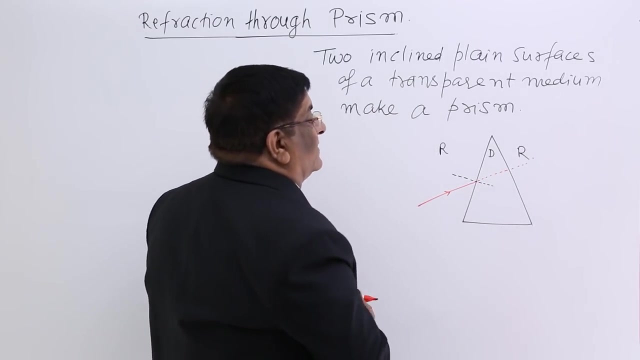 We draw a normal here, because this is the interface. This is rarer medium and this is denser medium. This is the normal medium, This is the barometer medium, This is the. this is rarer medium. now, this was going in this particular direction. this will bend toward. 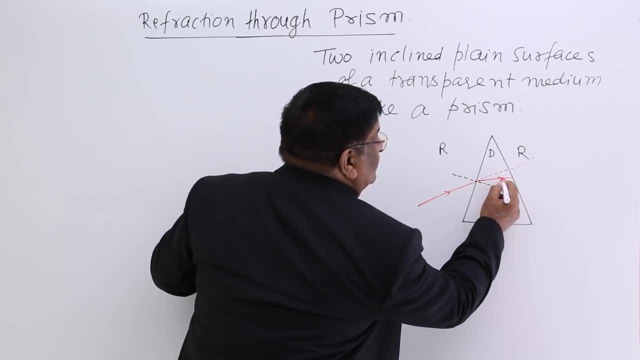 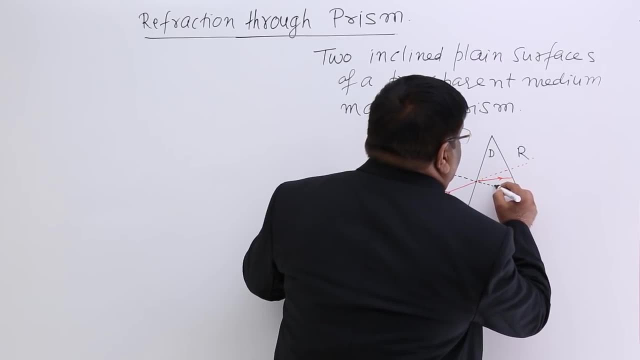 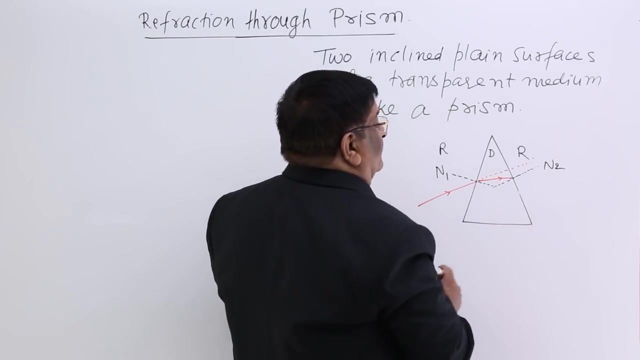 normal. so it bend toward normal. now it reaches this particular surface. here again we draw a normal. this is a normal of this surface and 2. this was normal on surface number 1. this is normal on surface number 2.. Now this ray which is going in this direction, there is a change in the medium from denser. 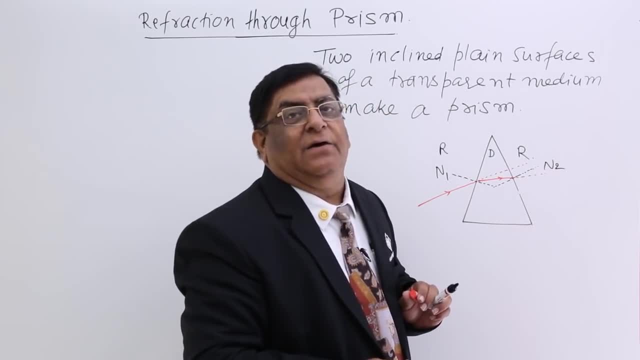 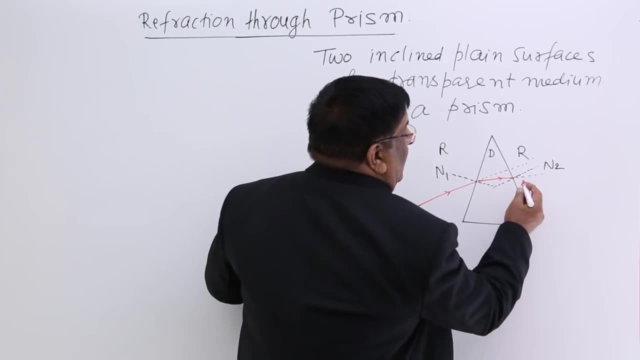 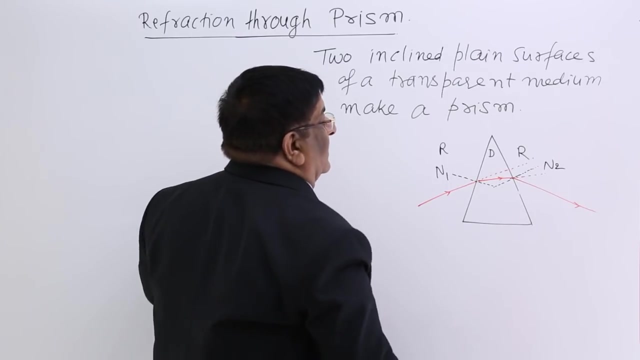 to rarer and our rule says it will bend away from the normal. this is normal, this is the original. So it will bend away from the normal and it will go like this. so this is the path. there is one refraction here, there is another refraction here, but the shape of prism is cut in such 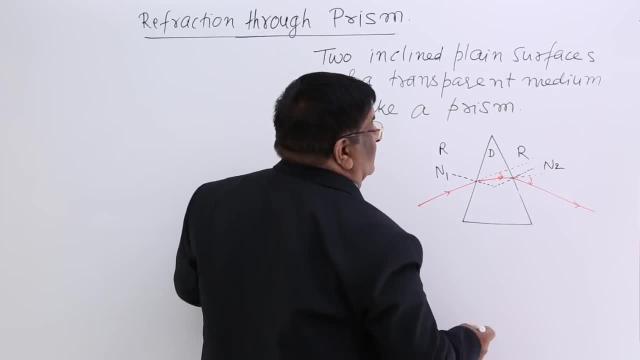 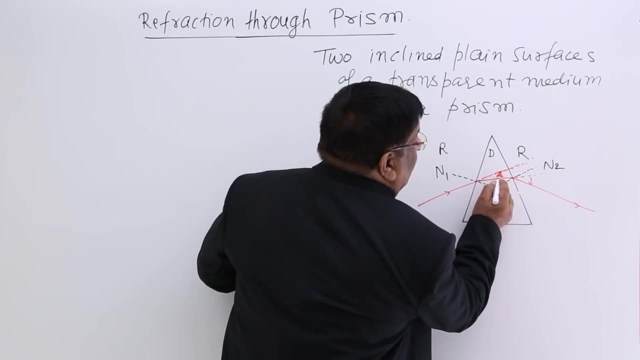 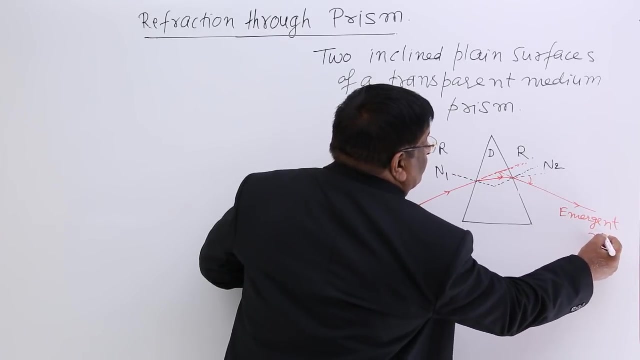 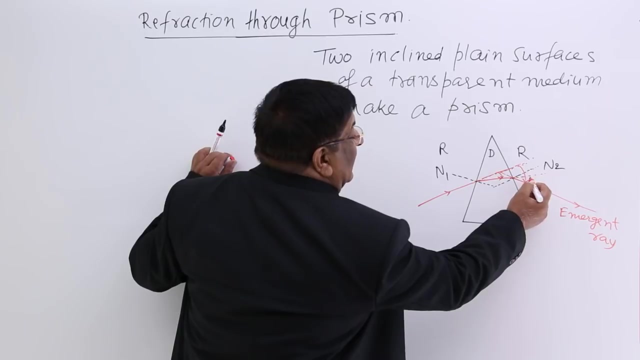 a way, that effect of both the diffraction is that it ultimately see this was the very original path And this is the final path. this is emergent ray, the ray which is coming out, and from the original path there is always certain angle. this is in comparison to the original ray. 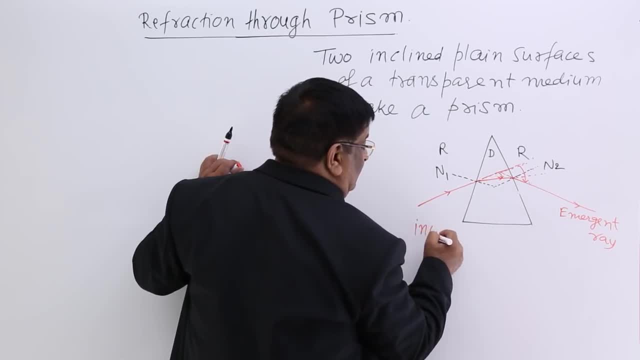 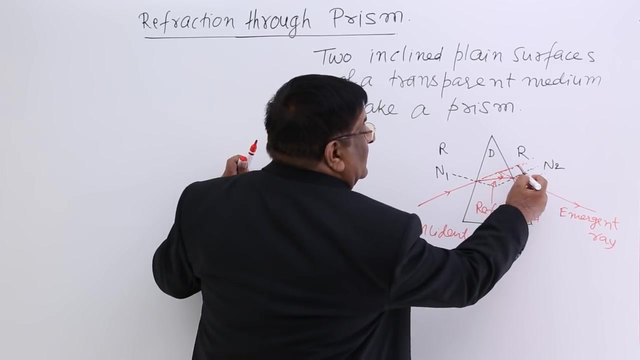 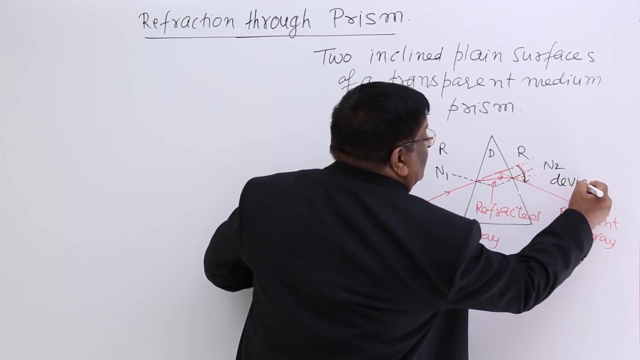 not this ray, This is incident ray, This is refracted ray, This is the final path, Refracted, And this is emergent ray. The angle between this was the original incident ray and this is the final ray, the angle between the two. the angle between the two is known as angle of deviation. 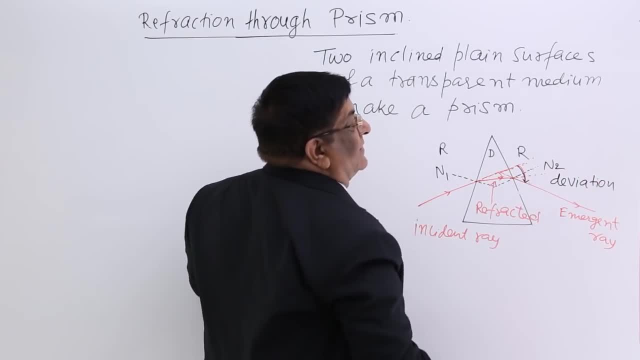 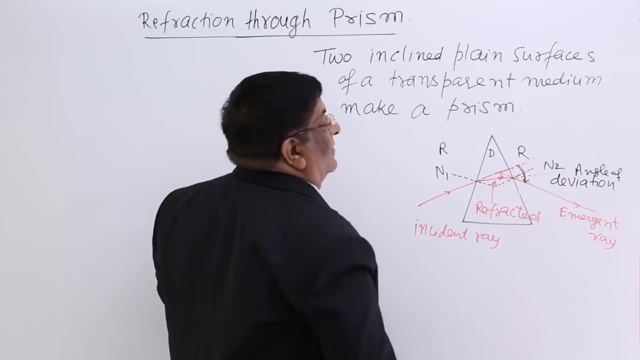 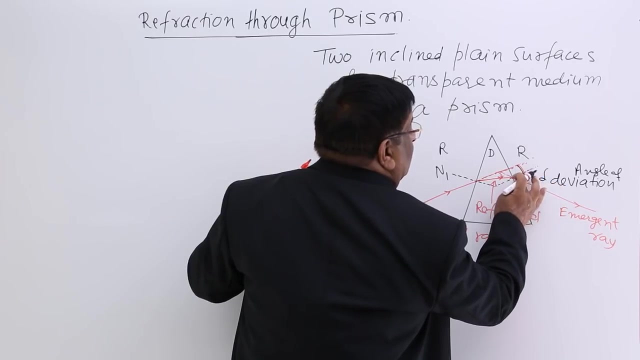 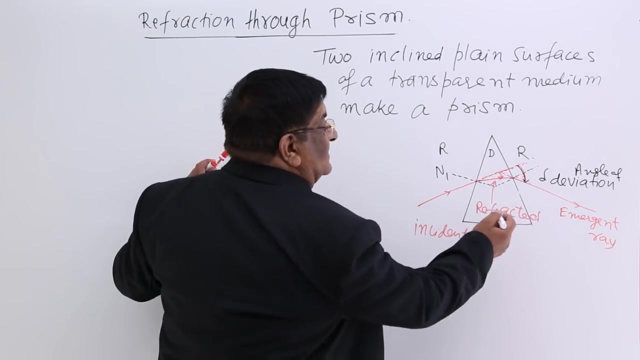 Because this is the deviation in the path. so this is Angle of deviation, Angle of deviation, Angle of duration, deviation, and we have in symbol for this, we call it delta. So delta is angle of deviation, original path, and this, This is a refracted ray. So this is angle of incidence and this 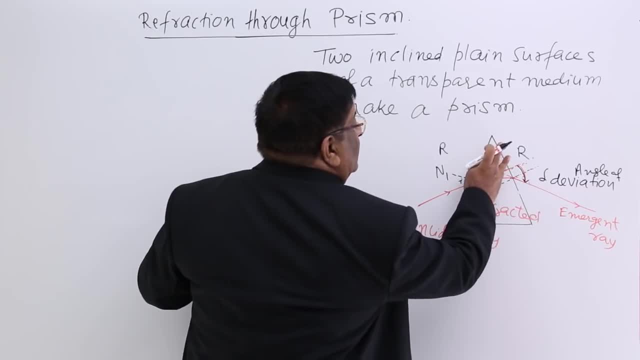 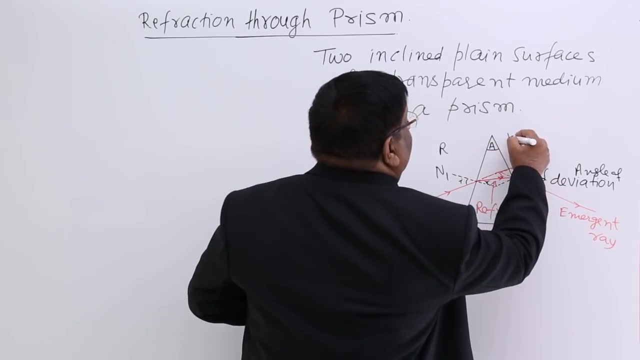 is angle of refraction. Now, these are the two surfaces which are involved in refraction. There is an angle of inclination between these two. This is a very important angle and this we call angle of prism. This is angle of prism. So this is general what happens So in prism. 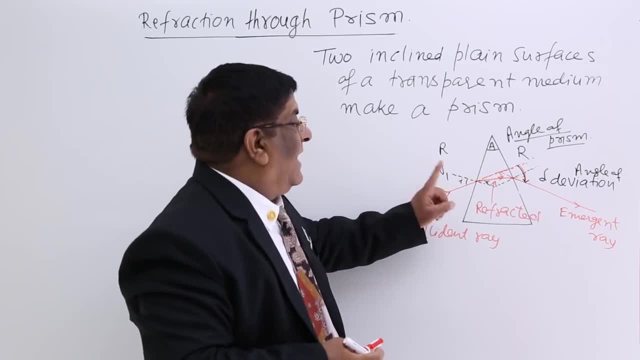 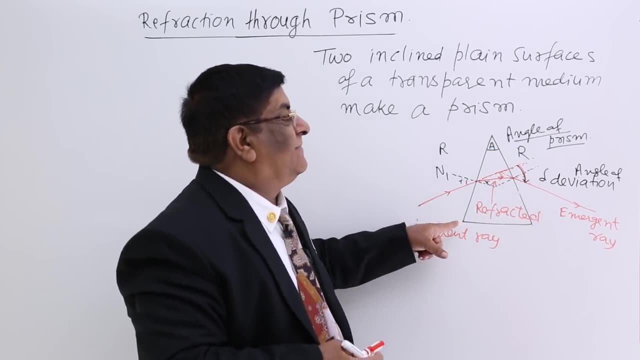 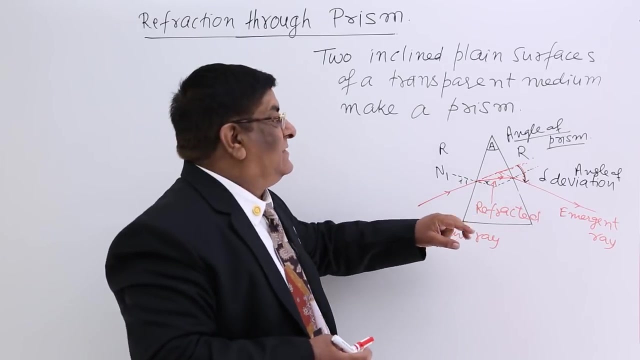 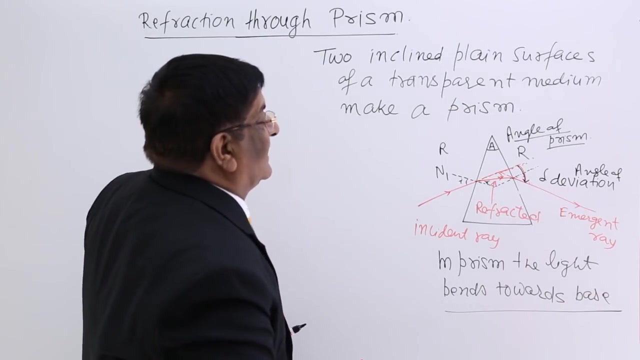 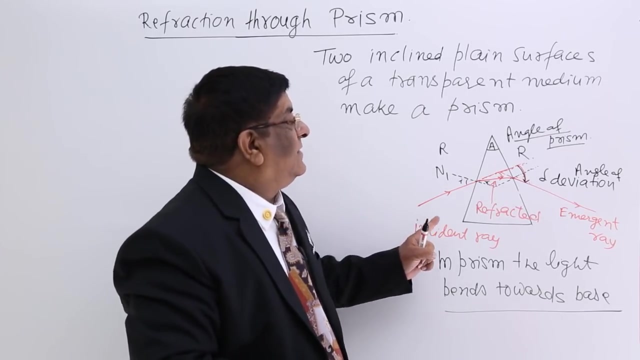 what happens in prism: A ray entering on one face is bent, is deviated, towards base. Remember what is the direction of deviation? The direction of bending. Answer: the direction of deviation is towards base. So this is what prism is. Now we have to establish relations that how much will be this deviation and this? 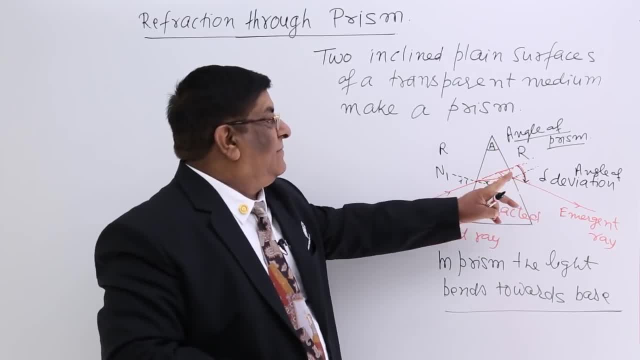 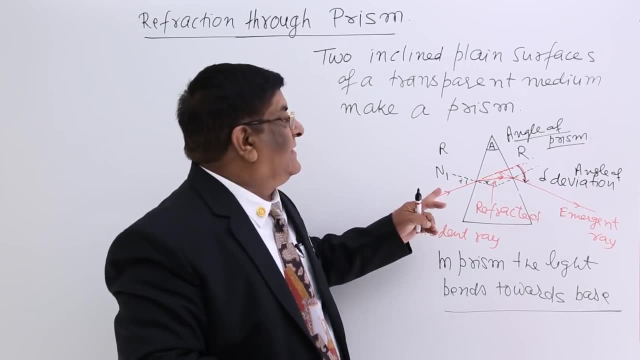 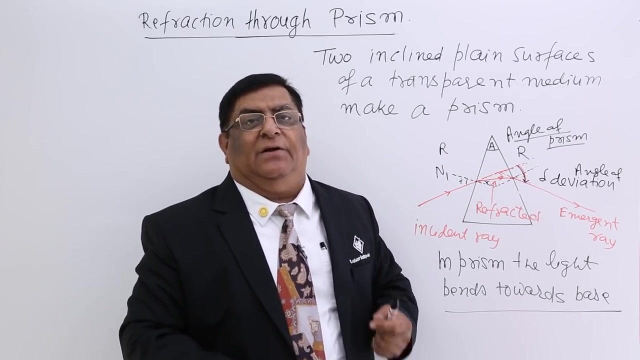 deviation is affected by what? Is it affected by refractive index of this material? Is it affected by angle of incidence? Is it affected by angle of incidence? Is it affected by angle of prism and any other quantity? So now we will make a relation and find out how much. 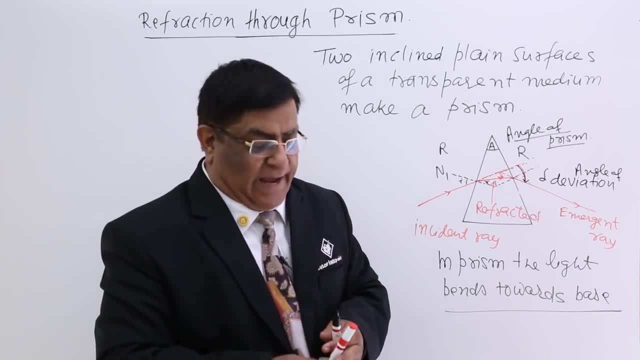 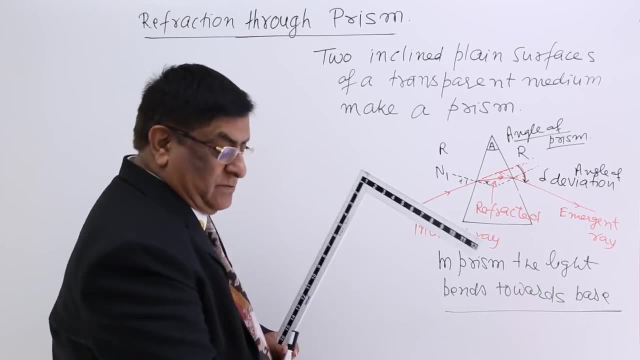 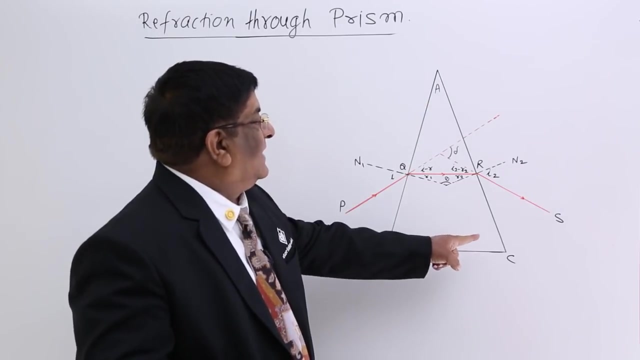 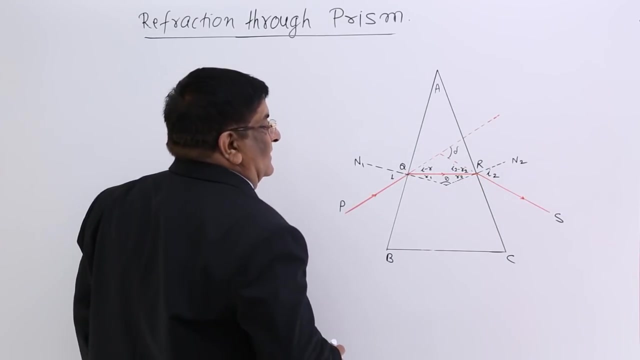 is the angle of deviation related to other angles. So I will make a large diagram of the prism. Now we will do certain calculations of the angles. a, b, c is section of the prism. This shows the path of the ray, which we have already discussed. 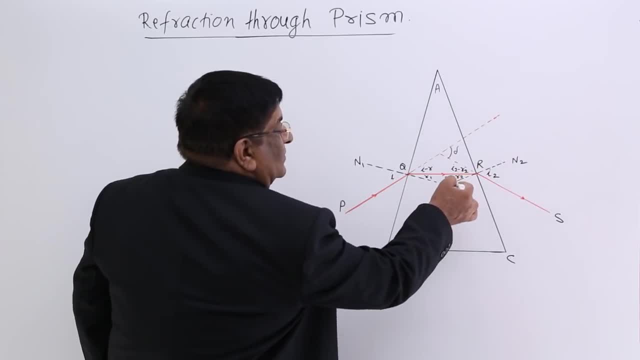 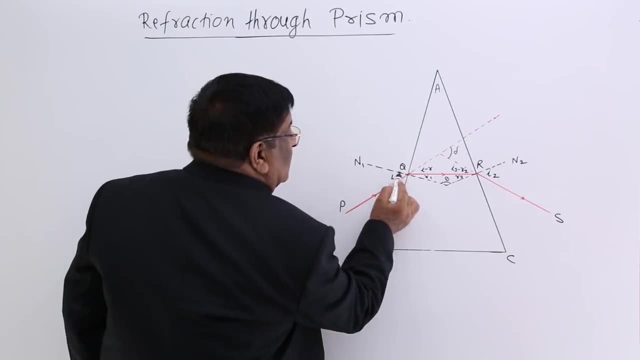 Now, this is normal 1,, this is normal 2, this is angle of prism A For the relations. this is a normal. this is a normal. it is a 90 degree. it is a 90 degree, 180 degree. 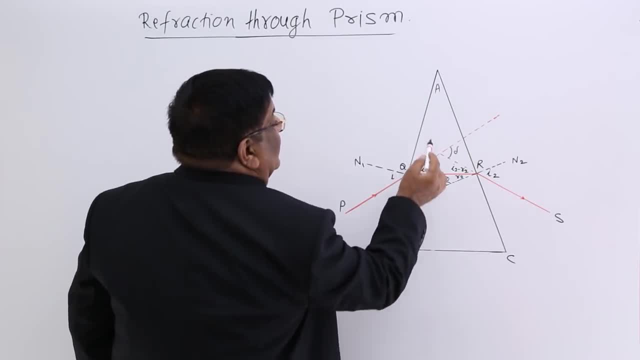 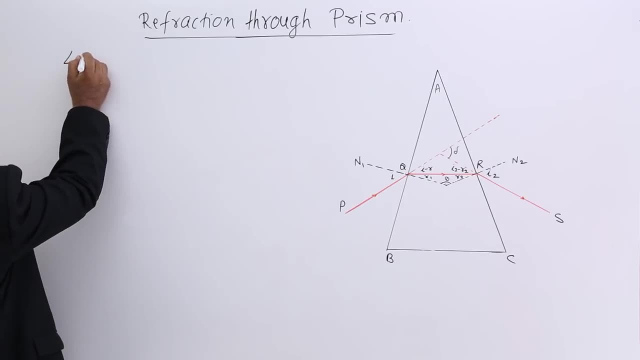 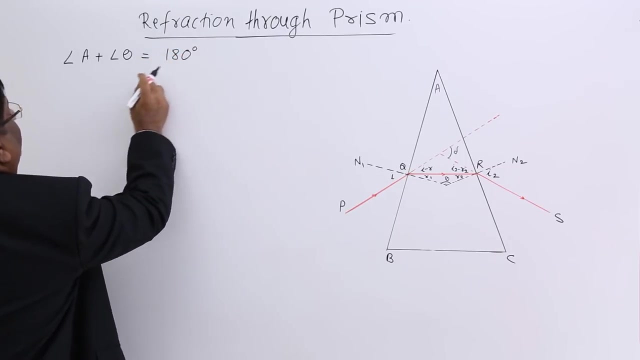 So sum of these 2 angles is equal to 180 degree. that is, A plus theta is equal to 180 degree. Angle A plus angle theta is equal to 180 degree. Now we will not write angles, just for the sake of simplicity. 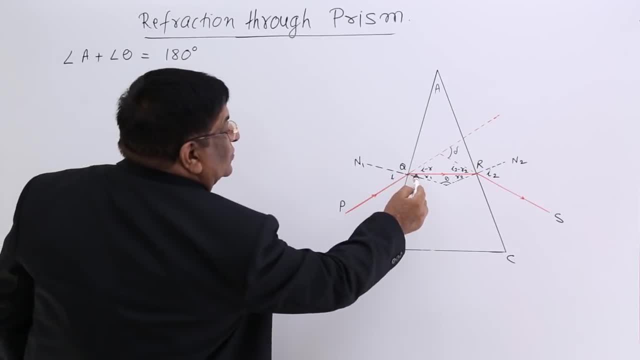 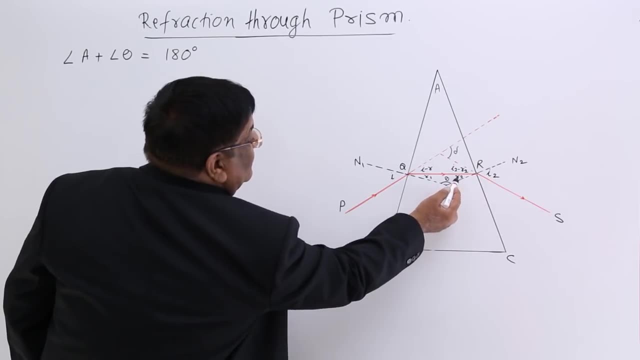 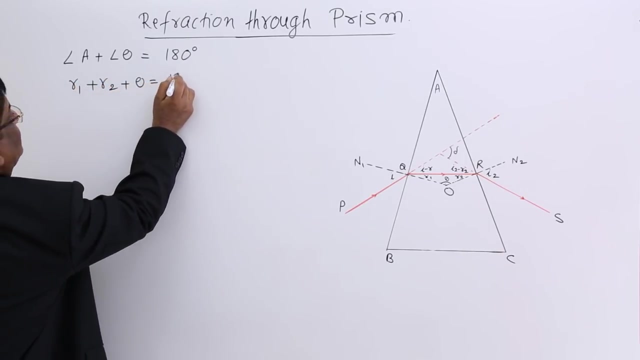 So we also know that in the triangle QRO, QRO, theta plus R1 plus R2 is equal to 180 degree. R1 plus R2 plus theta is 180 degree, And these 2 give us one result: that these 2 are equal. that means A is equal to R1 plus. 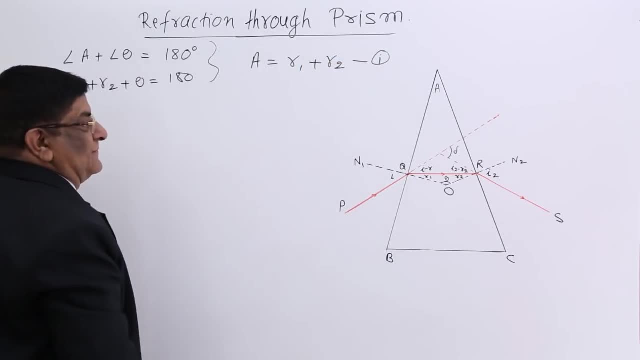 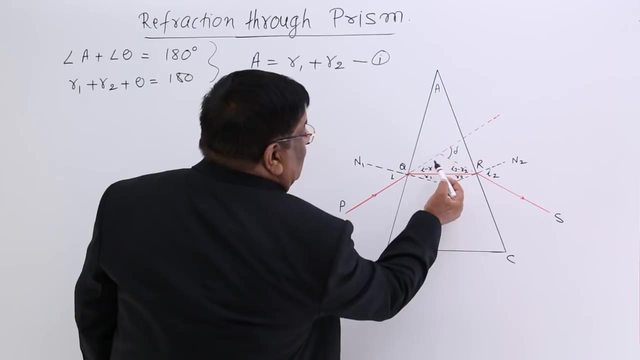 R2.. This is one result. okay, Now see angle A: Delta. this delta, this is external angle of this triangle, this triangle external angle. So it is equal to sum of these 2 angles, That is, I1, R1, I2, R2.. 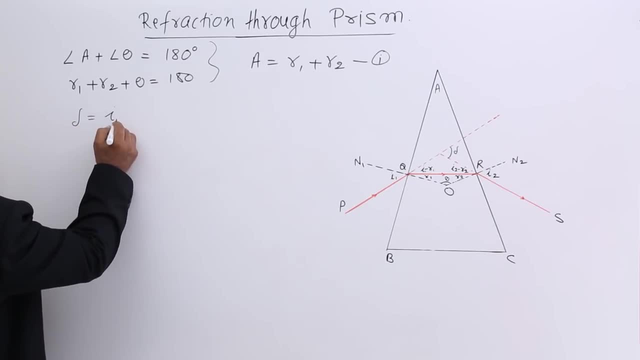 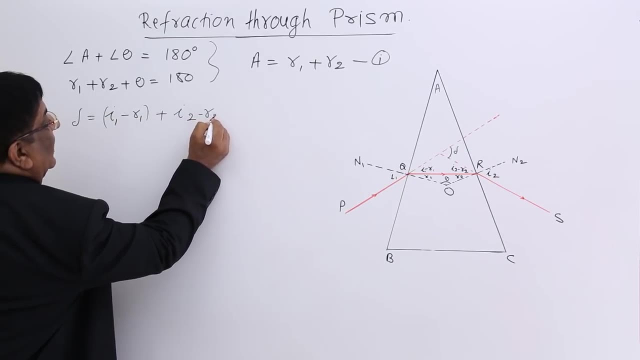 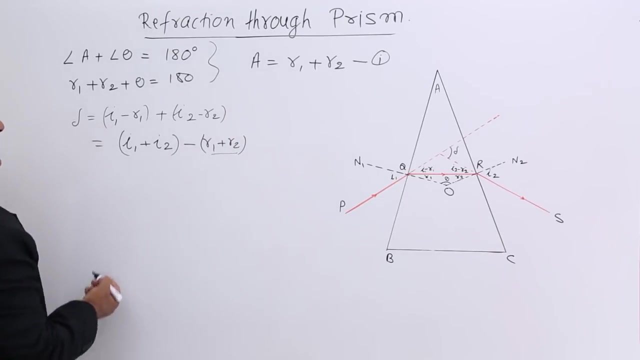 So delta is equal to I1 minus R1 plus I2 minus R2.. Okay, So this is it, Thank you. Or we can say this is I1 plus I2 minus R1 plus R2.. Now this R1 plus R2 is equal to A. 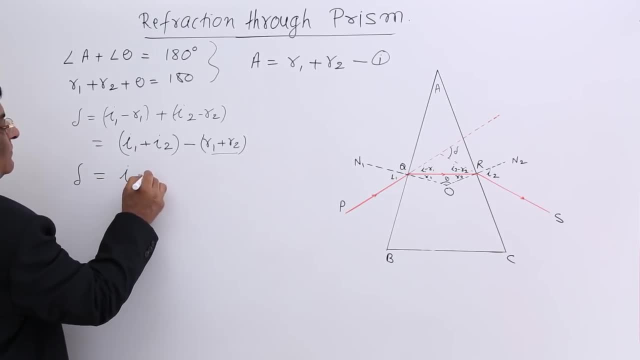 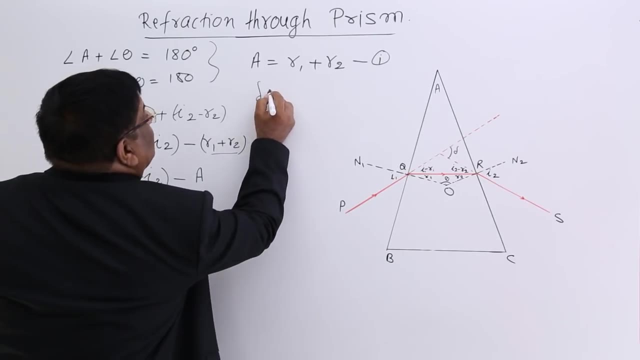 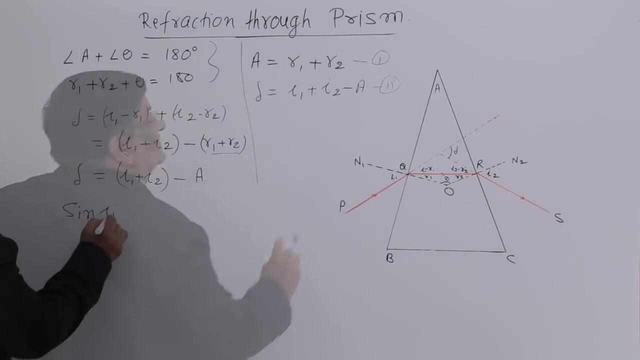 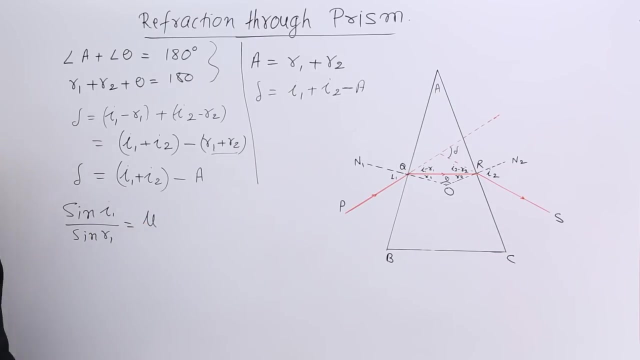 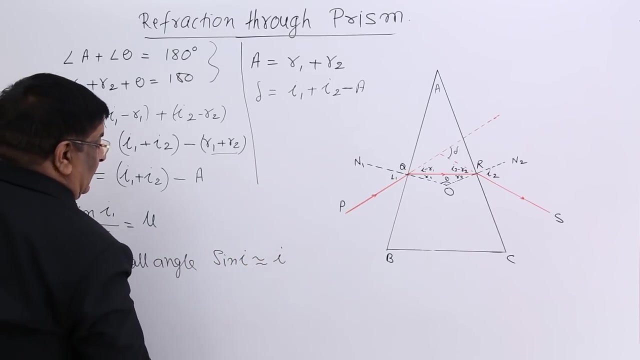 So delta is equal to I1 plus I2 minus A. So delta is equal to I1 plus I2 minus A. This is another relation. Refractive index is mu, that is, sin i upon sin r. For small angle sin, i can be treated equal to i, So we can write it as: i upon r is equal to mu. Therefore, 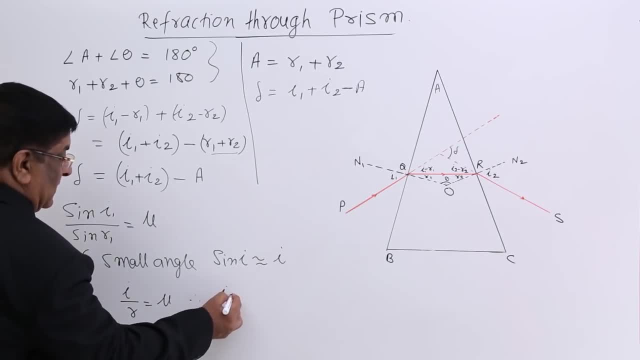 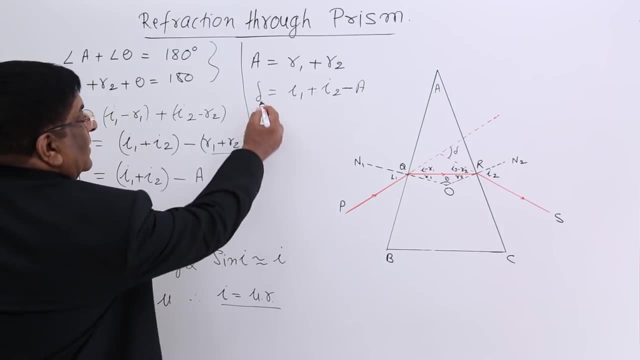 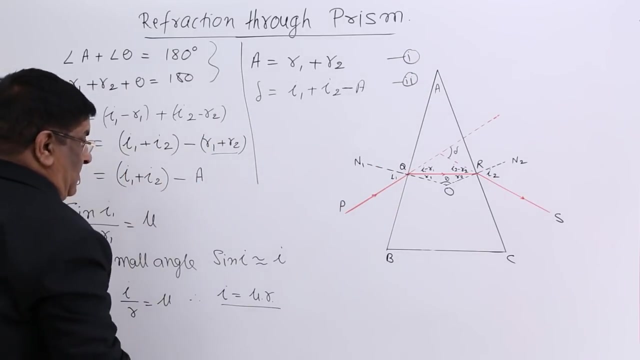 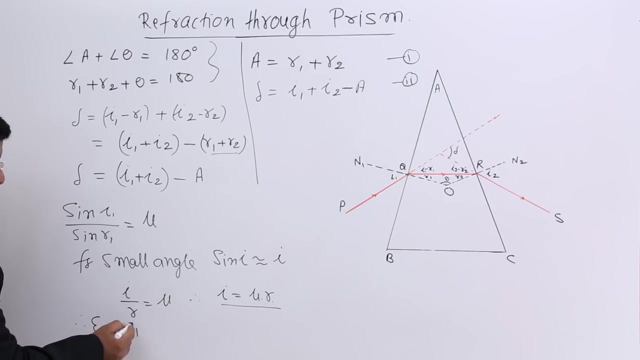 i is equal to mu into r. So from equation number 2, therefore equation 2,, delta is equal to I1 plus I2.. mu is equal to I1 plus i. Our lets also say mu is equal to mu into r1 plus mu, r2 minus. 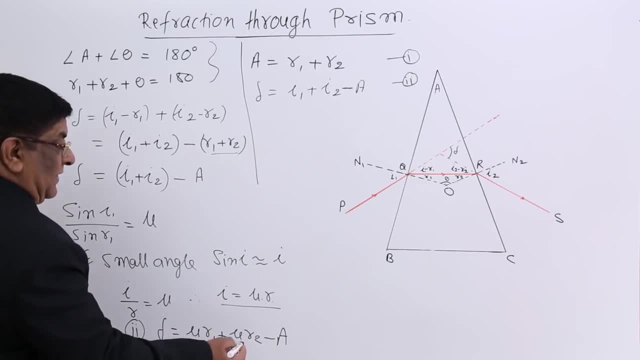 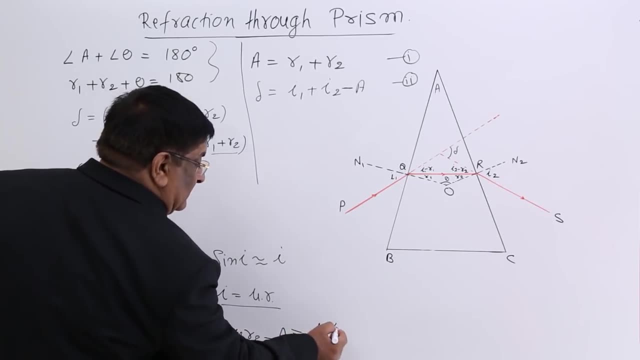 a. Now, out of this we can take out mu as common mu and this will be r1 plus r2, r1 plus r2 minus a. but we know r1 plus r2 is equal to A, So I will write it here: delta. 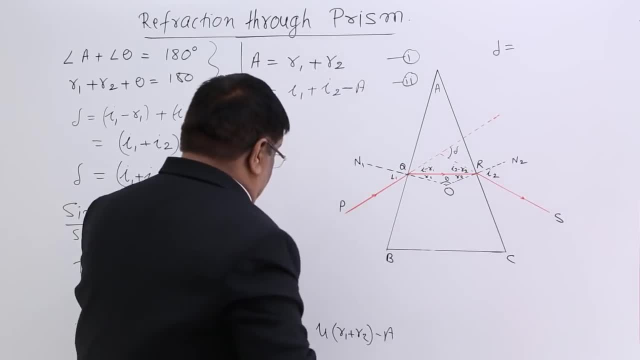 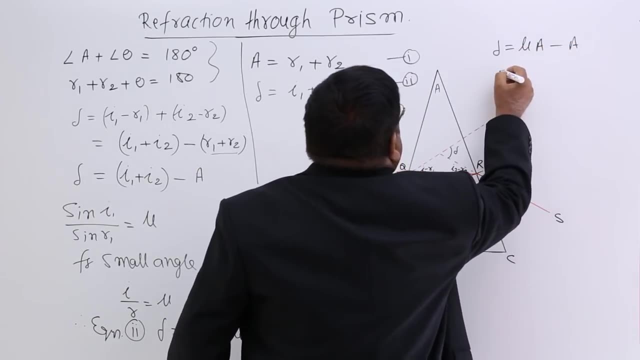 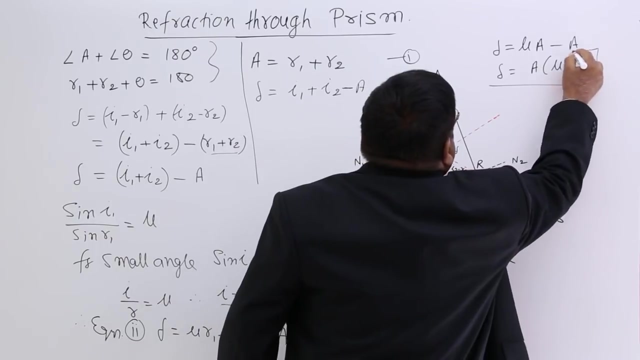 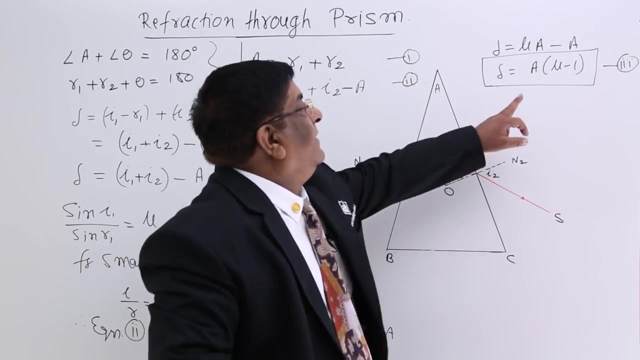 is equal to r1.. I1.. I2.. to mu into A, mu A minus A. So delta is equal to A mu minus 1.. This is another important relation. This is relation between refractive index A and delta. This is only delta angle. 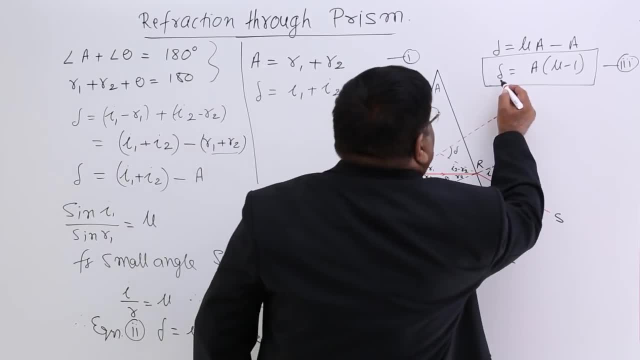 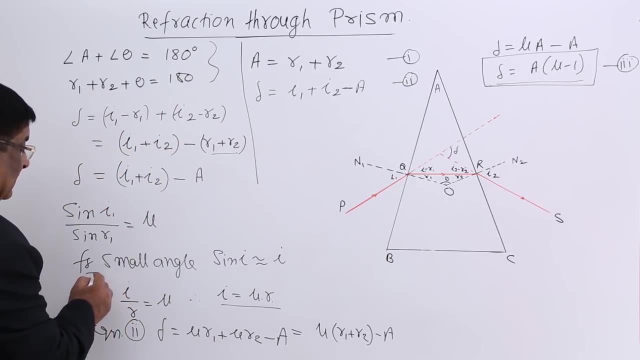 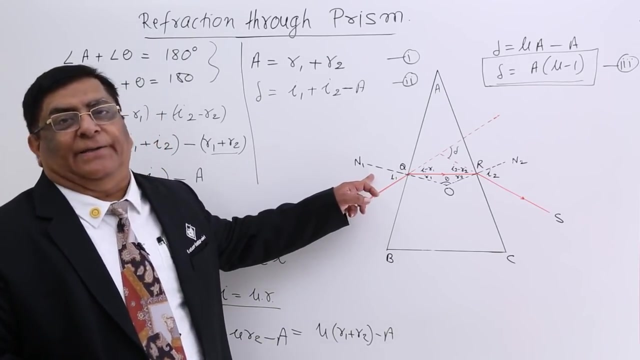 of incidence and A. So this is a very important relation. but for this relation you should remember something, that is this: It is true only for small angles and not for all the angles of I. When we take large angles of I, this relation does not hold good. So for 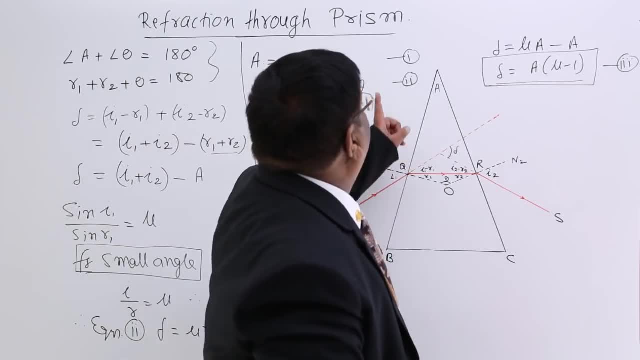 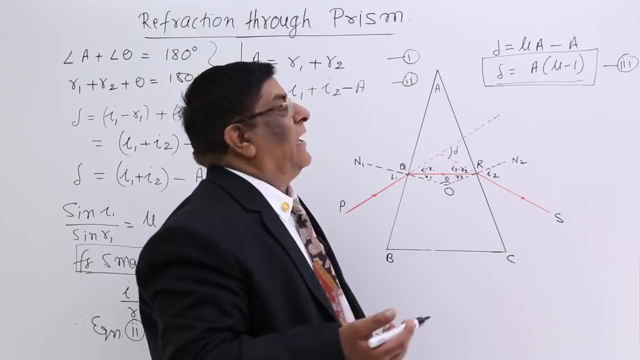 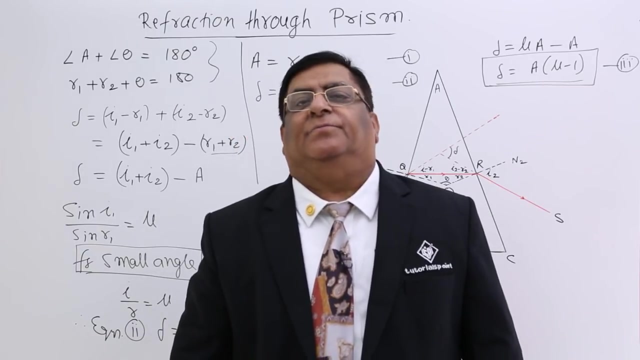 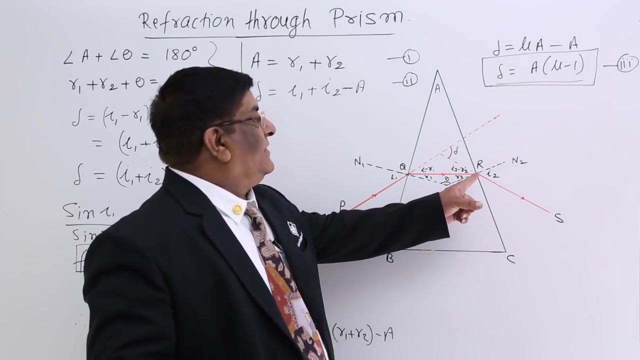 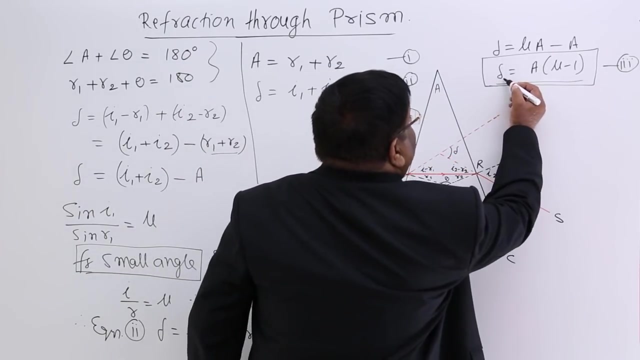 small calculations. this is okay. So we remember these three formulas and R. after that we do certain Bohr calculations And those calculations are. there is a particular condition in the prism that is known as minimum deviation. This deviation you are seeing here, this deviation, This angle depends upon what This angle depends upon: refractive index N. 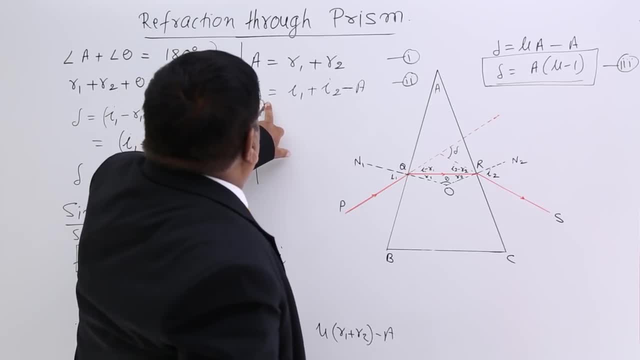 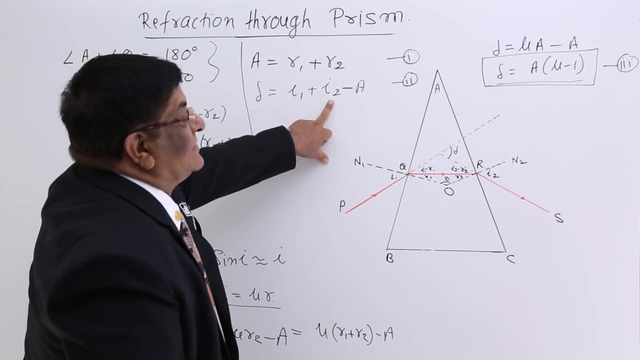 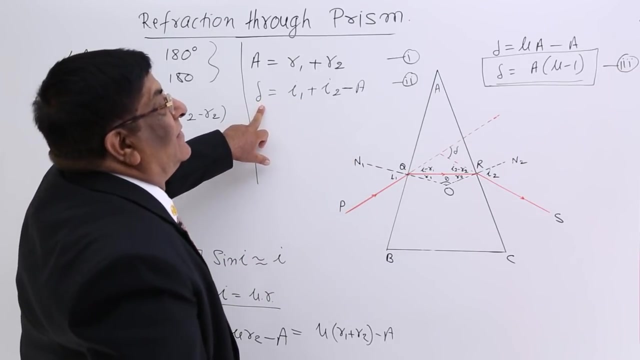 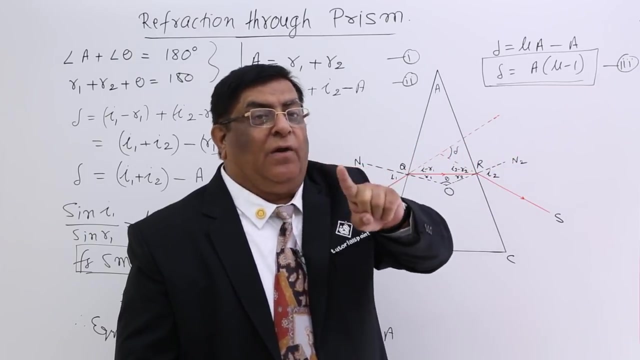 this A, But this angle also depends upon angle of incidence and angle of this emergence and these angles may be different. In that case delta will be different. So delta is not constant. It is constant only for a very small angle. I This will be constant, But for small values. 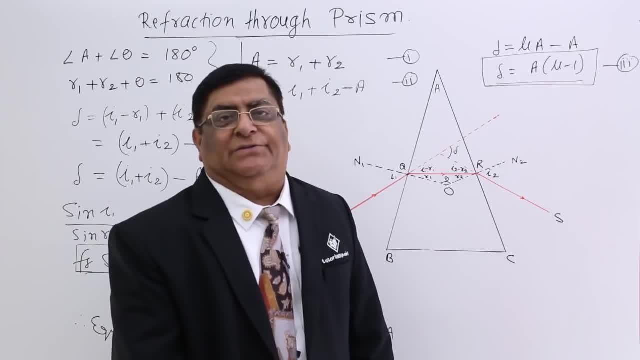 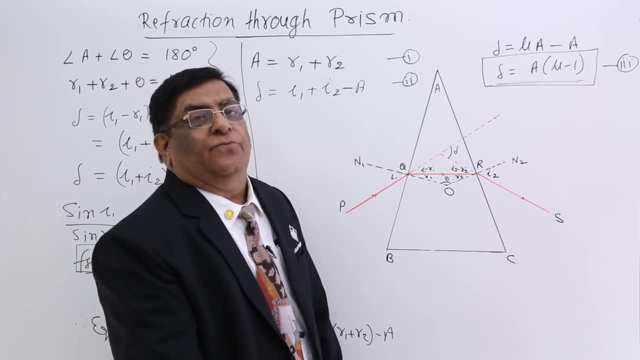 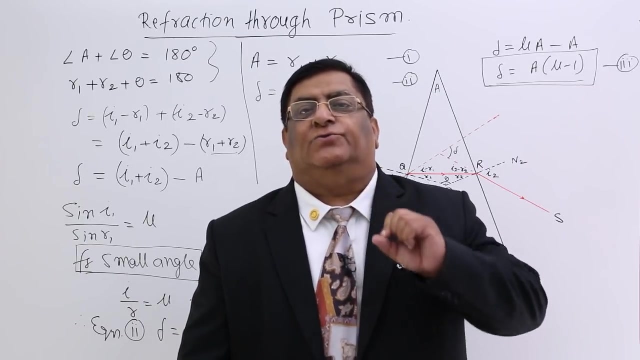 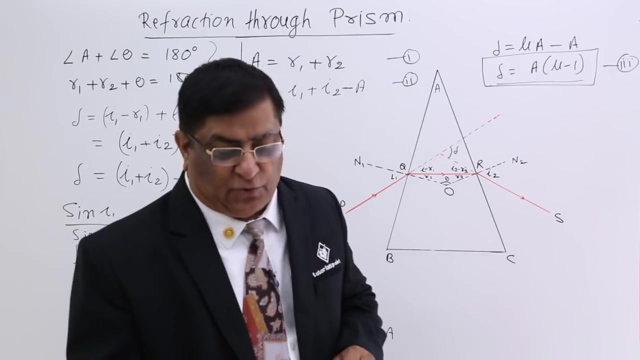 that means for large values. this may change And now we will study how delta will change with respect to I. So we draw I and delta relation for different values of I and we see how delta varies when you are varying I. So we do another type of experiment. We haveату dakika nya. i. so latitude at this time. alpha1 ka delta, value delta. We are doing some kind of previous experiment, day 2 or day 3 experiment which is simplyураungِّ or nabing nabaningh冒at imallowaby. Sometimes we do these, Sometimes this method will not. 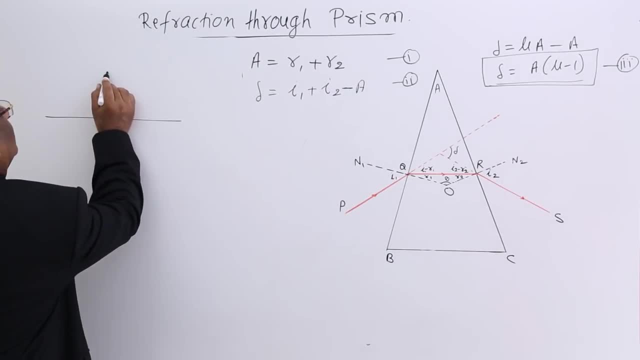 work, and now we have i過來, delta to delta. So delta is normal. relative to delta exists between. Draw a line and on this draw another line as perpendicular. Now draw a line which indicates direction of incident ray. this Now put a prism at this place. 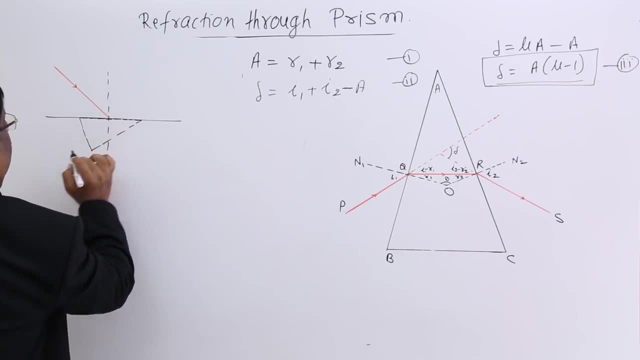 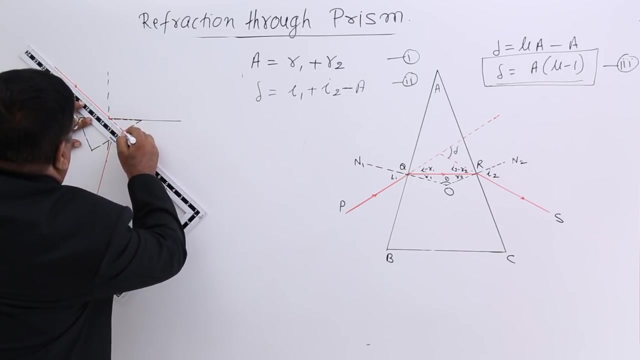 This is a prism. Now, what happens to this ray? Answer is this: will enter the prism And go out of the prism in this direction. This is path of it. Where is the deviation? This is the deviation. This is the deviation. 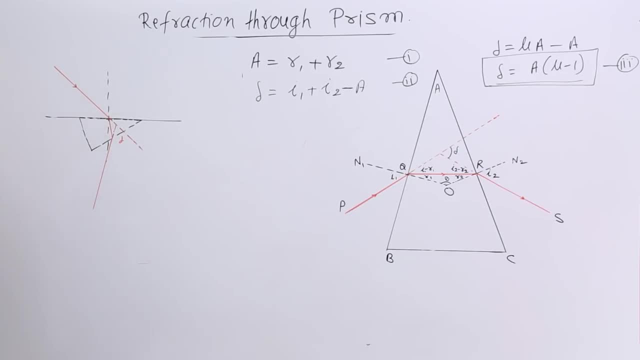 This is angle of deviation. Now we are doing it in the lab. We take a prism, put it on this line, make two pins here and see without prism, put two pins more. Again, I tell you: two pins, no prism, two pins more. 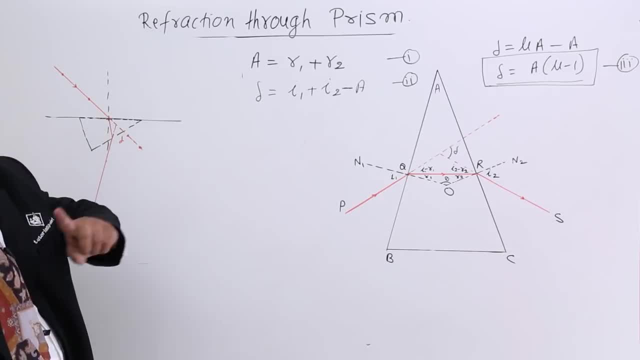 This gives the angle of deviation. This gives the total direction of the ray. Then we are placing one prism here. After placing, we see these two pins and we see that one. these two pins are in line, appear to us in this direction. We put two more pins here. 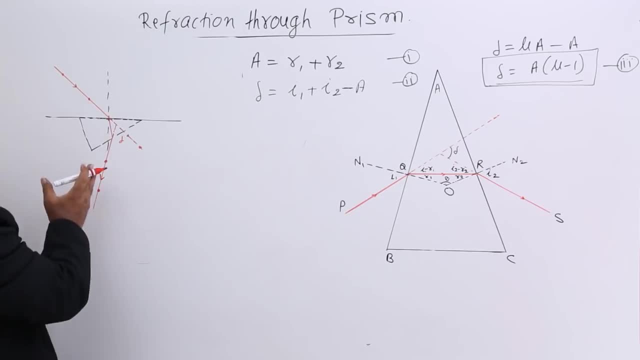 This shows the ray. Yes, When we see through the prism, We put our eyes here, We put our eyes here. When we put our eyes here, we don't see the pin. We put our eyes here, don't see the pin. 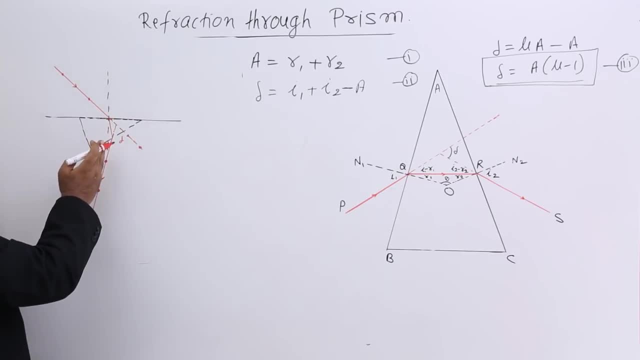 We put our eyes here, we see the pins As if they are placed somewhere here This way. So we draw, we put these two pins before this and draw the line. This is the direction of outgoing ray. Now take out everything. 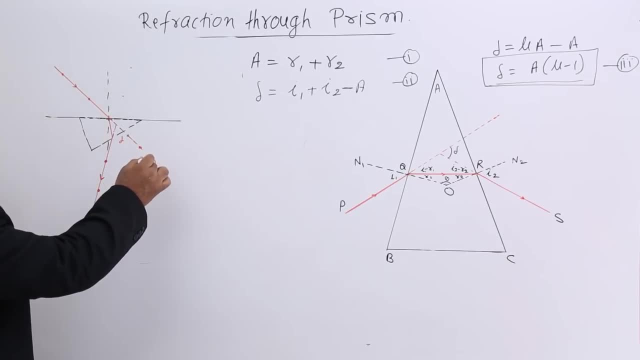 Mark the line. This is the line of incoming ray, This is the line of outgoing ray and this is the angle delta. and here is the angle i. We take the reading of the two, marking it as i1 and this is delta1, and then we make: 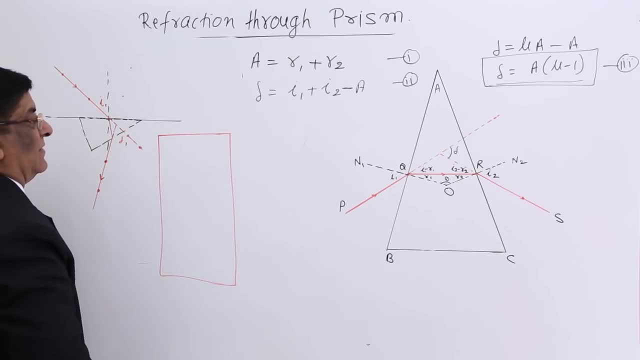 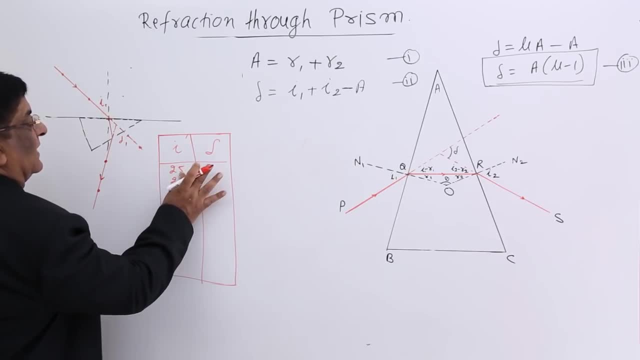 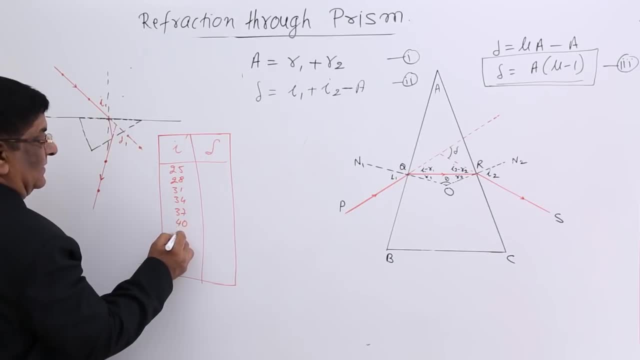 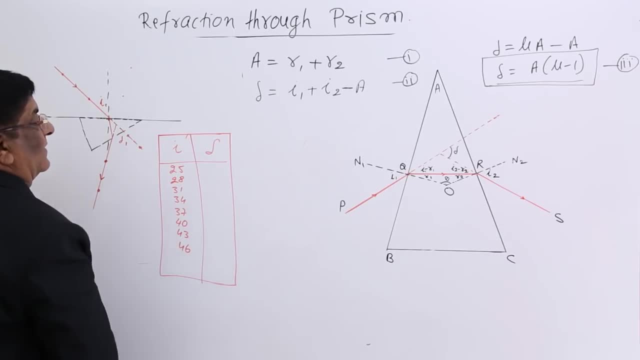 This is the angle out the value of delta, and it comes to like 50 when this is increasing, this goes on decreasing. this is 50, then this is 48,, 45,, 36,, 35,, 38,, 40,, 46. see the peculiar behaviour incident. 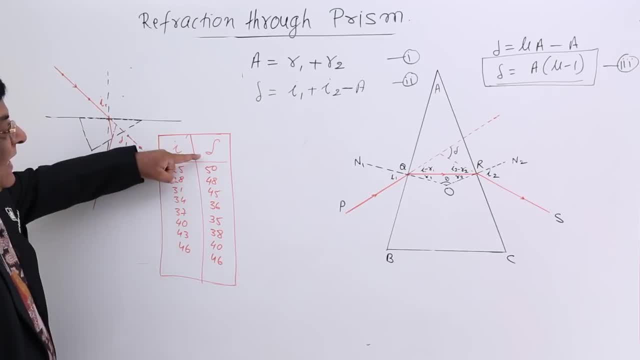 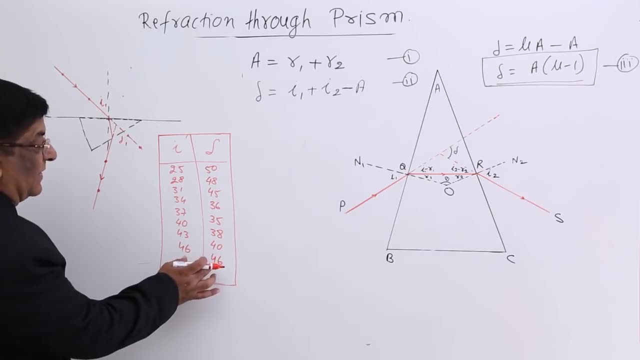 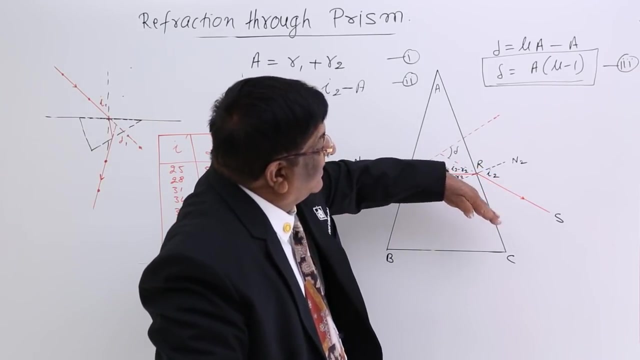 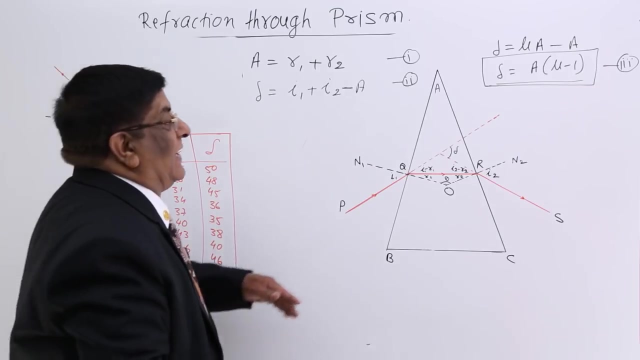 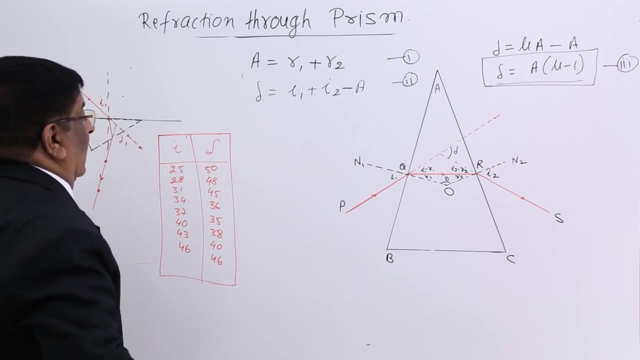 angle is increasing continuously, but delta. first it was decreasing And then it was increasing. this is the behaviour of delta. that means this angle was first increasing and then it was. first it was decreasing and then it was increasing again. first it was decreasing and then increasing again. this is the behaviour of delta. 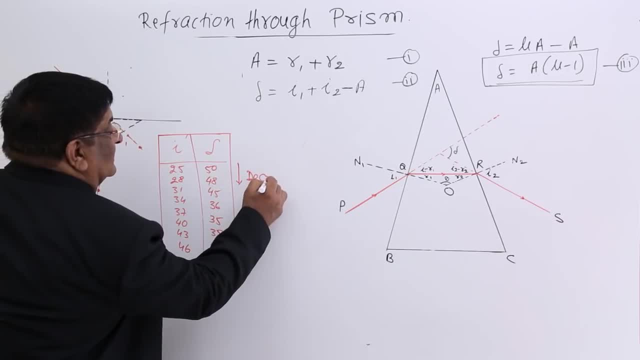 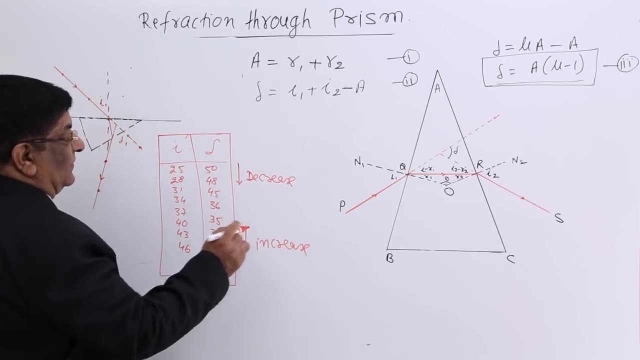 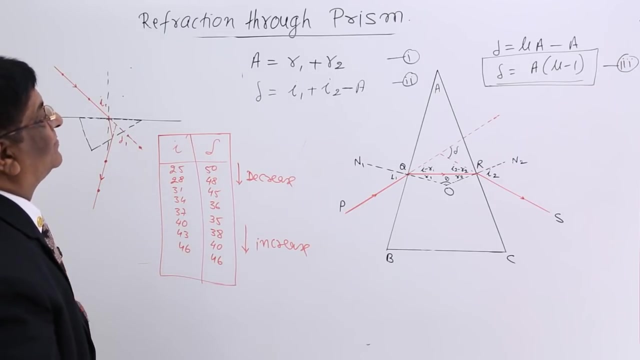 So this you remember decreasing and then increase, decrease, then increase. If we want to show it in a graph, that is a very important, very peculiar graph. we see, and the graph is like this: This is delta and this is i. Now we put different value of i here and we put different value of delta. 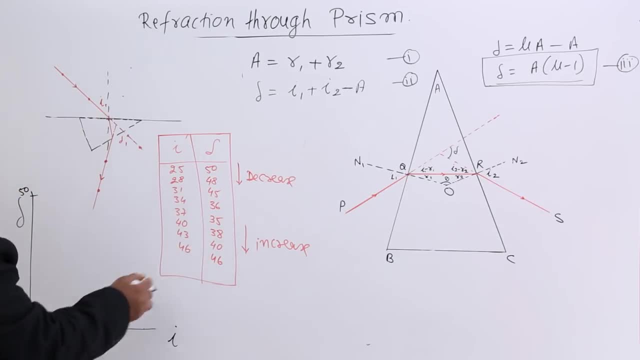 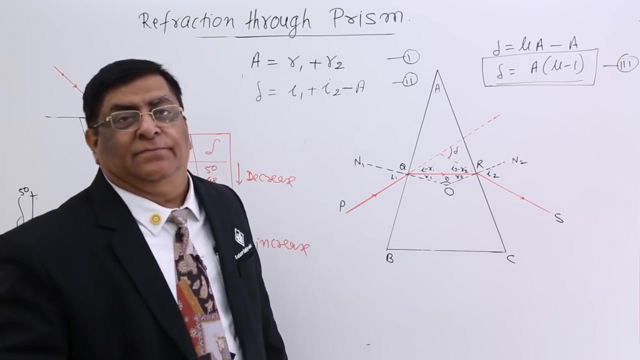 here, Let us say, 50, and here it is 30. So 50,, 48,, 45, and this goes on increasing. So we get the points like this this way. Now, when we join all these points, we are supposed to join them in a smooth curve and 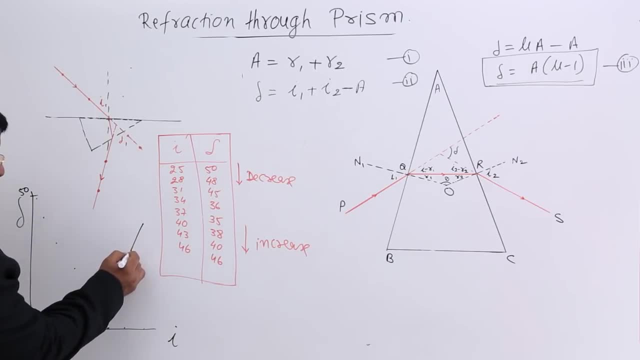 not in the line: line, line, line, line. This is the wrong way of joining them. How we should join them: First, put all the points this way and then we will join them in a smooth curve. Now I will join it for you. We should make it. we should try to make a smooth curve. 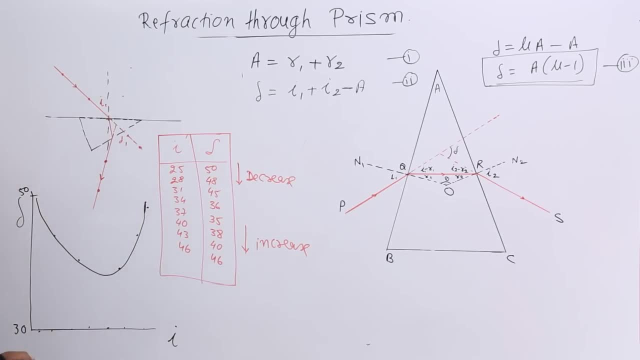 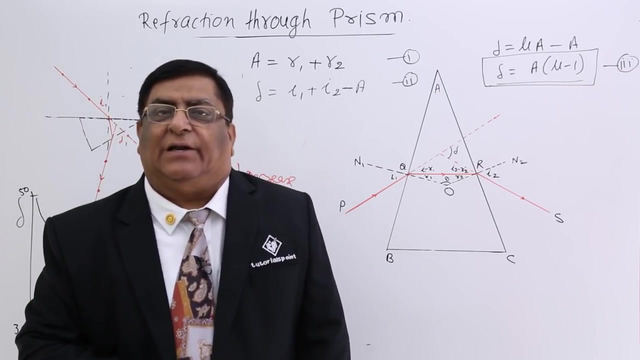 That is like this: It is quite likely that some points will be slightly inside, some points may be slightly outside, does not matter, Let it be. But what is our target? that the the graph should be a smooth curve, This smooth curve, and to make it a smooth curve, you will. 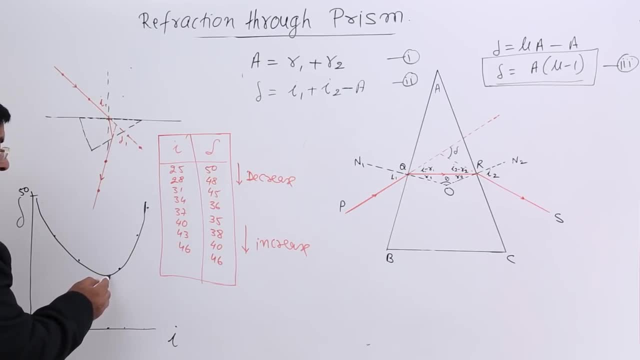 find that the bottom of this smooth curve has always come below these dots. That means if we say every point has one value of delta, then this bottom most point, this represents the minimum value of delta. We call it delta m: minimum value of delta for a particular 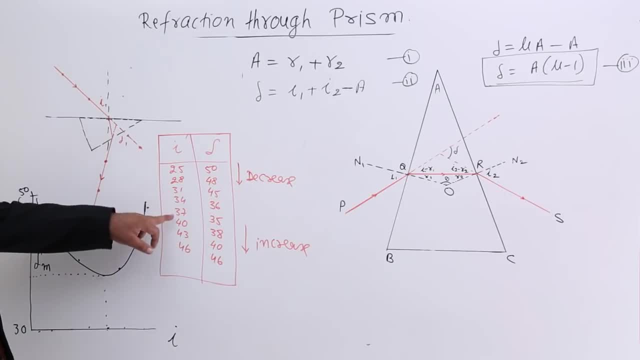 value of i May be for this value of i. we have not measured delta, so we have missed the minimum value of delta. That is why we draw this graph and with help of this graph, we find the minimum value of deviation, what is possible with the given prism. 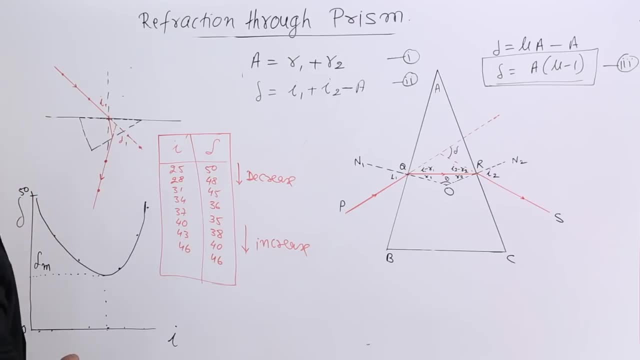 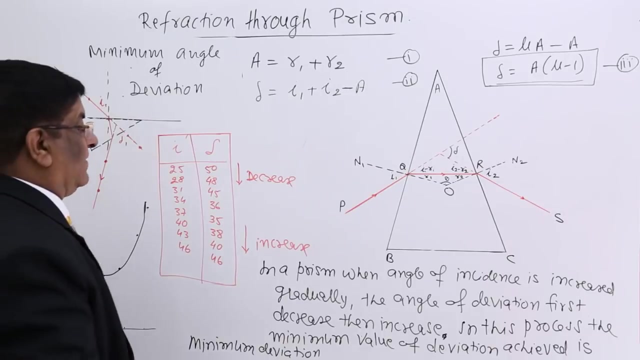 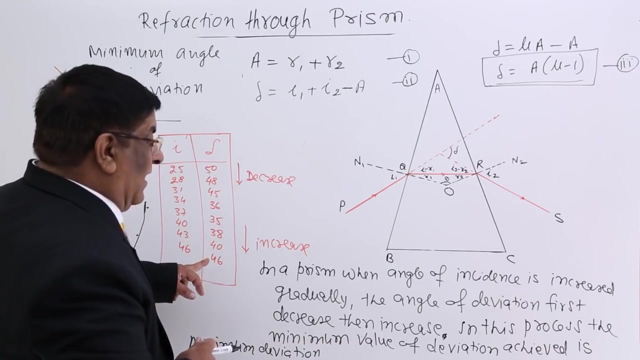 So this is how we get minimum angle of deviation. So what is minimum angle of deviation? Can we write it in the text? Answer is yes, We will write it this way. See, in a prism, when angle of incidence is increased gradually, the angle of deviation first decrease, then 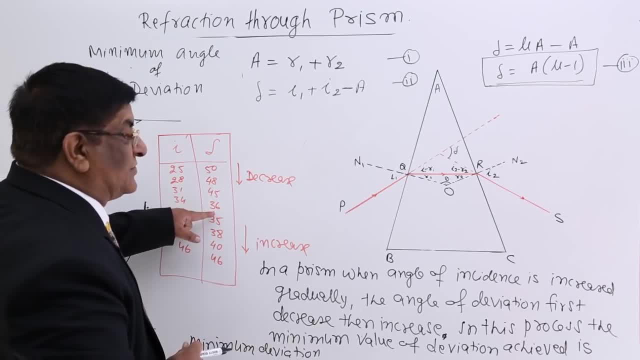 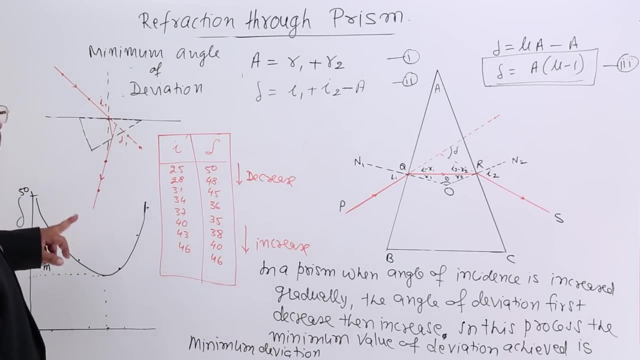 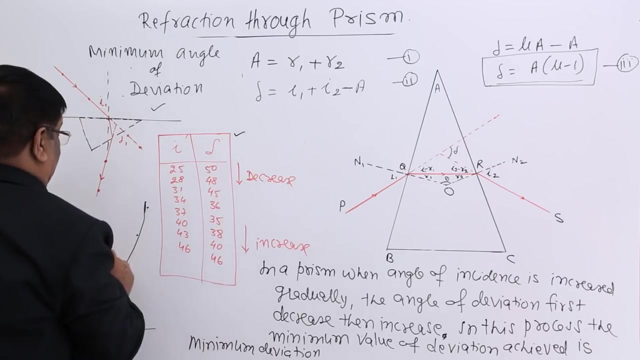 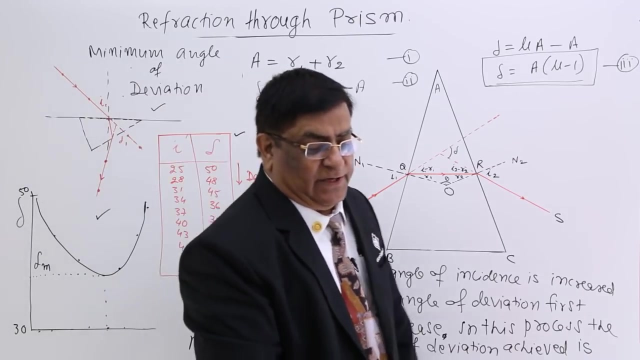 increase 1: 1 In this process. the minimum value of this of deviation achieved is minimum deviation through that prism. So when you are writing about minimum deviation, please make this diagram, make the table, make this one, and this gives the minimum deviation. Now, what is the use of this minimum deviation? And 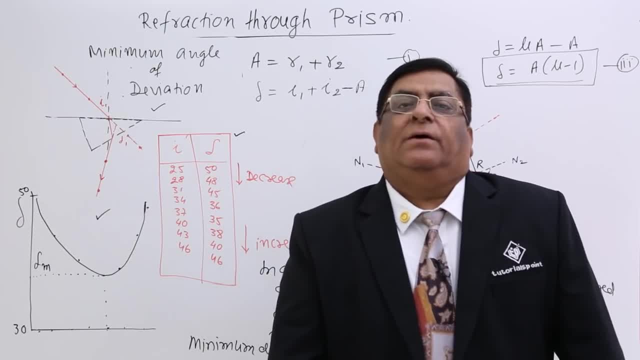 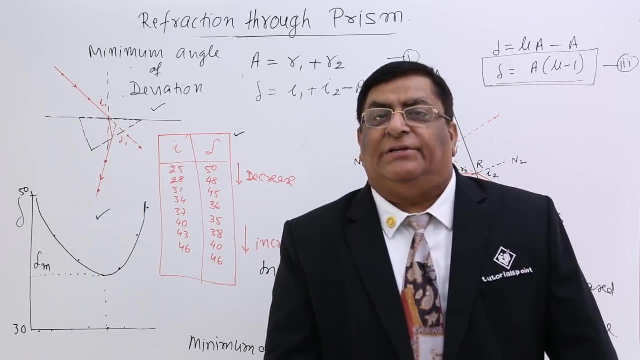 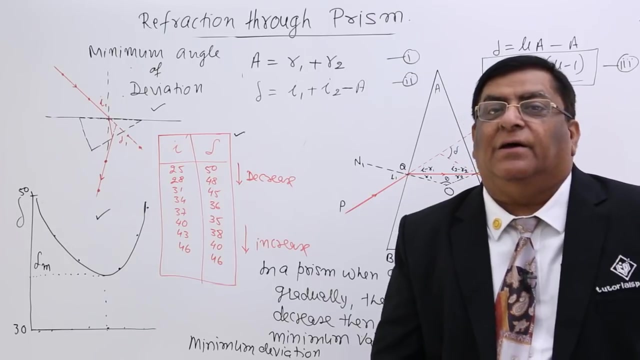 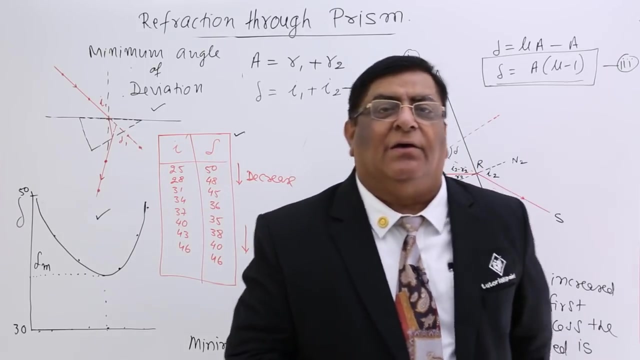 the next point is very important: When a prism is in the condition of minimum deviation. when a prism is in the condition of minimum deviation, we find that angle of incidence. i1 and i2 become equal to each other. Similarly, R1 and R2 become equal to each. 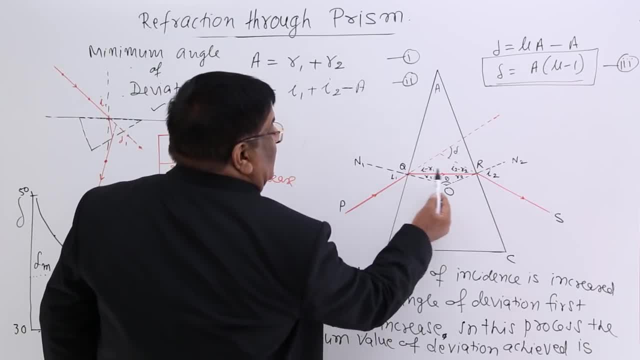 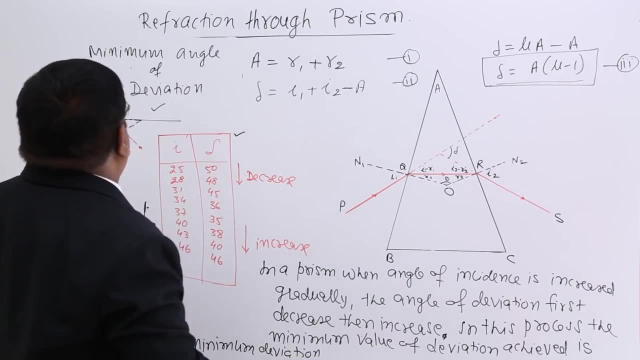 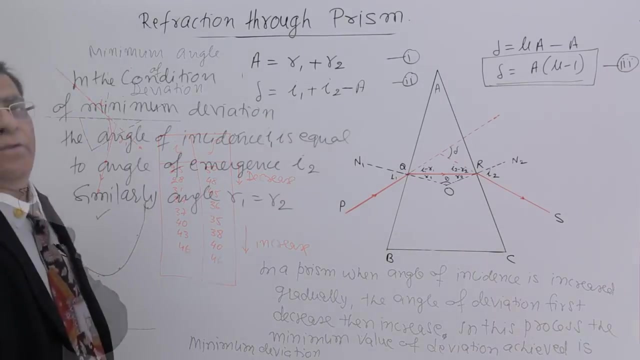 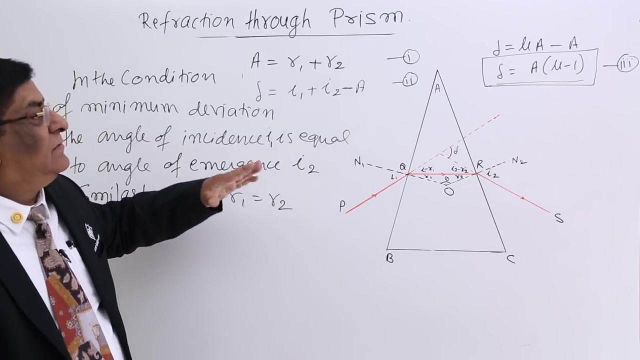 other I2 become equal and R1 and R2 become equal to each other. So now we can write the effect of minimum deviation. This you have already noted, so I will rub it off. At the time of minimum deviation, the conditions become such a way: the symmetry is so much that this I1. 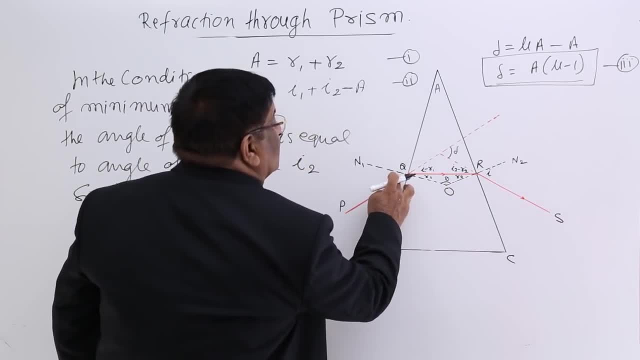 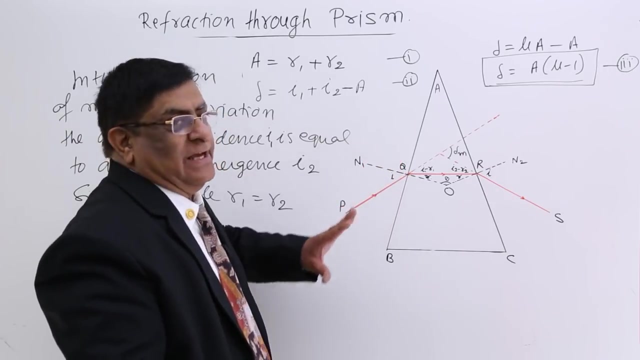 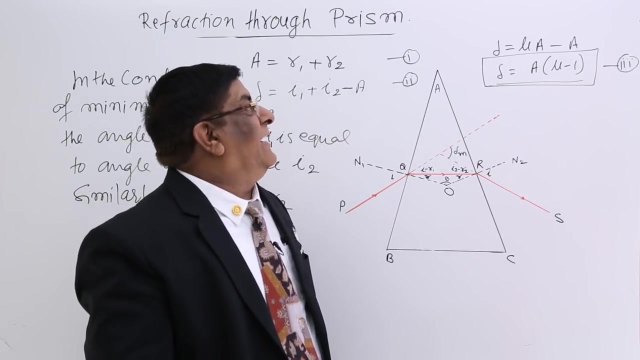 is equal to I2 and both can be treated as I When this delta is delta m and these two are R, R, This is R, this is R. Now, when this situation is there and we set the present for this situation, we have found the value of delta m. At that time we do our calculations. 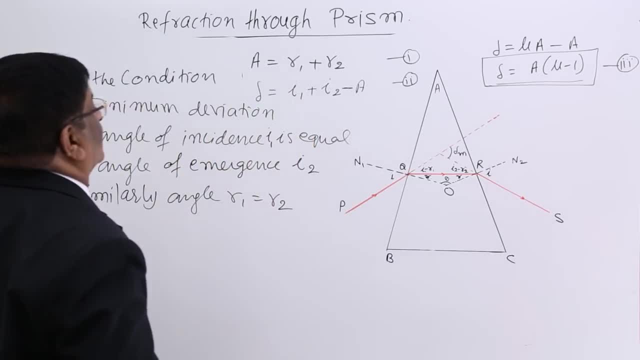 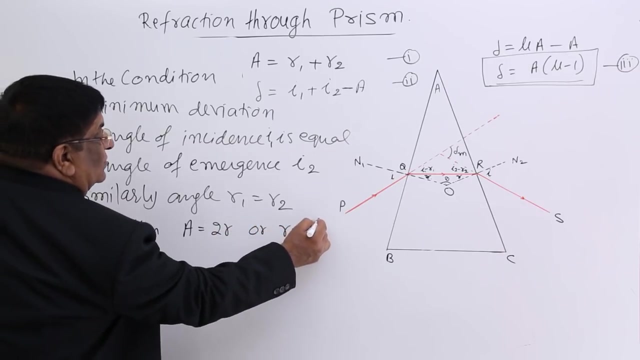 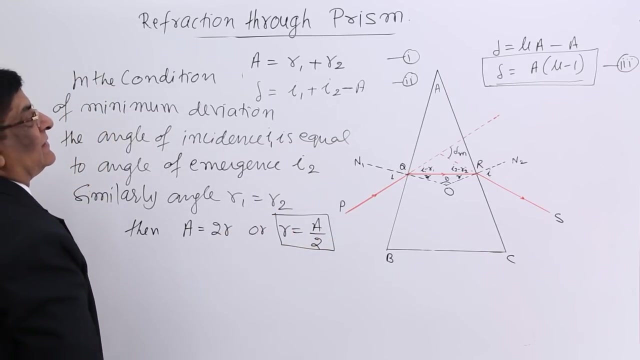 once again. And what are those calculations? Those calculations are from here. Then A is equal to R plus R, that is 2R, or R is equal to A upon 2.. This, The other result, is. other result is about the: I. This is. I, this is. 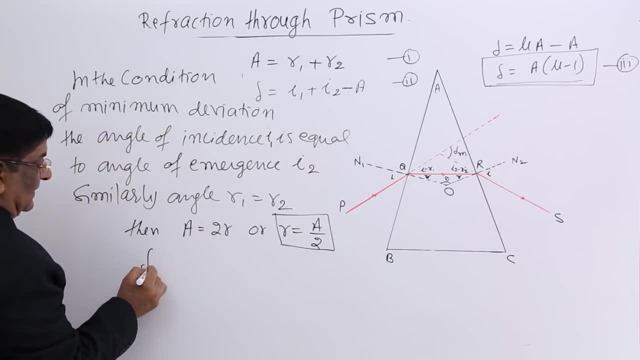 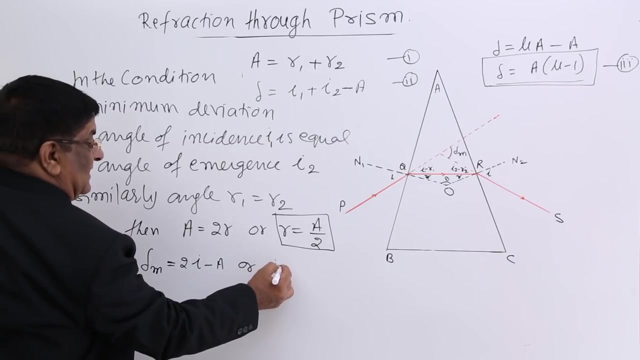 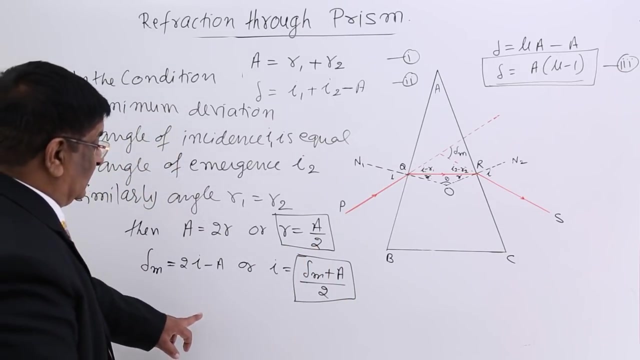 I, 2I minus A Delta minimum, because it is only at the minimum condition. delta minimum is equal to 2I minus A. or I is equal to delta m plus A divided by 2. This Now, with this, we can write this: 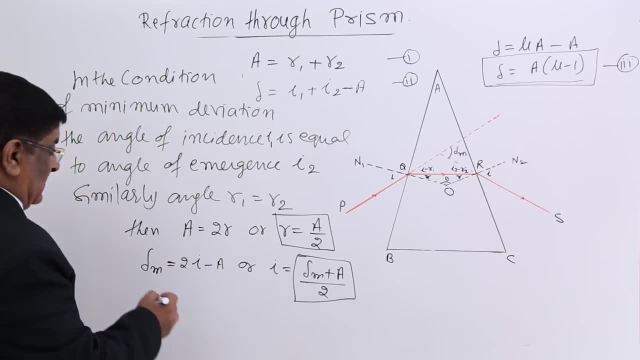 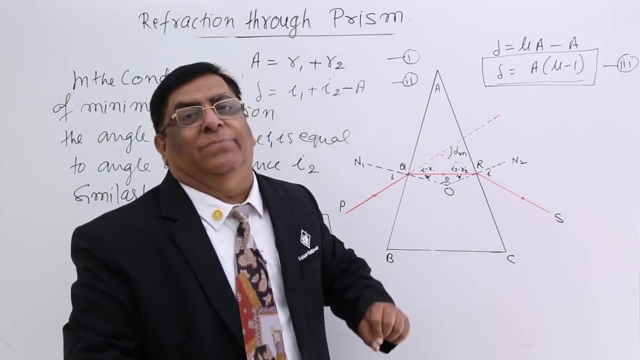 value of refractive index. Refractive index mu of the material of the prism is sin I upon sin R. Now we know the value of I in terms of delta A and 2.. Why we want to replace it? Because these are the angles which we can measure in the lab. in the laboratory We cannot measure. 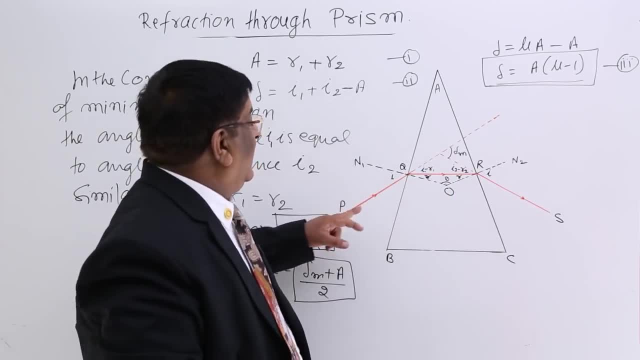 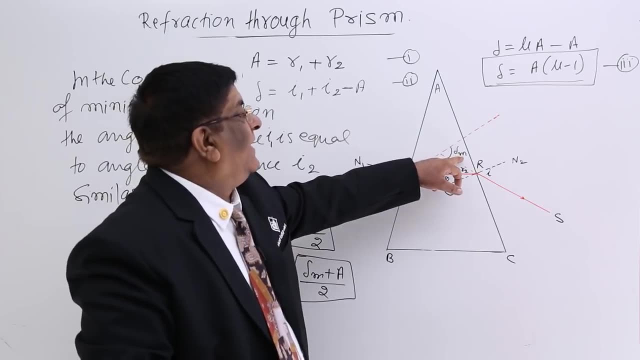 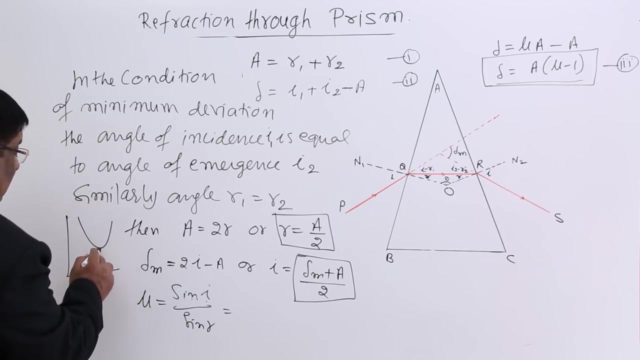 I R and this angle, But we can draw this line, we are seeing this line and we can always extend them to find this delta M. So this we can measure, we have taken it through the graph. this delta M we have measured. 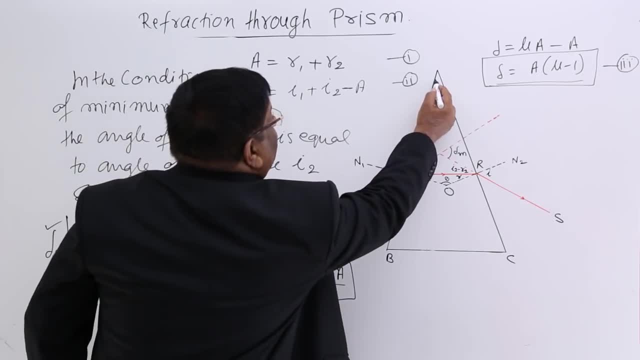 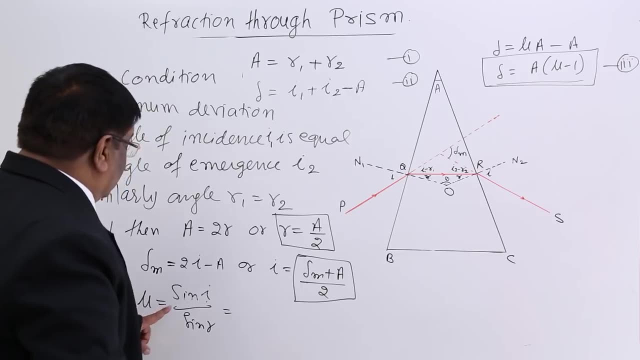 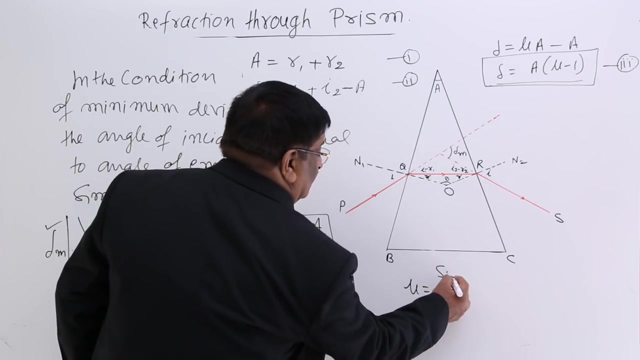 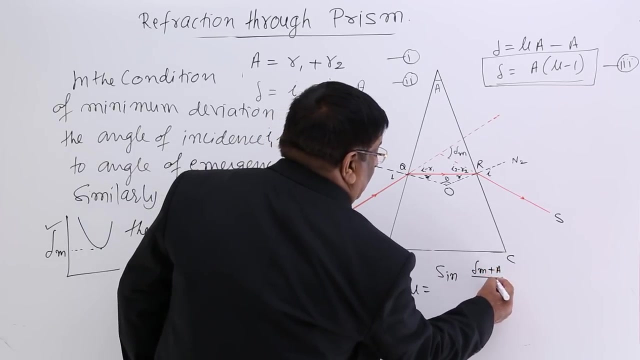 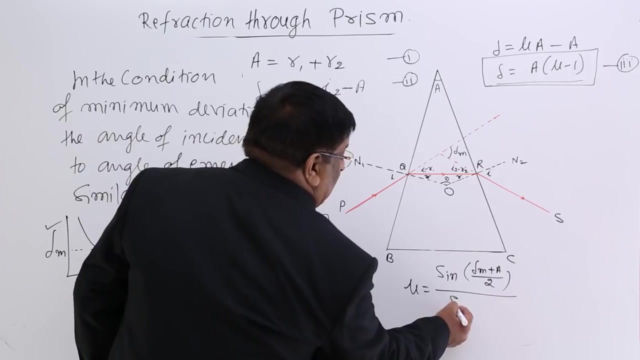 So this is a known quantity and A we can always measure here by drawing these two lines or by other optical methods. So mu is equal to sin i upon r. this we can write as mu is equal to sin. in place of i we will write this: delta M plus A upon 2, this is to be divided by sin r, sin A by 2.. 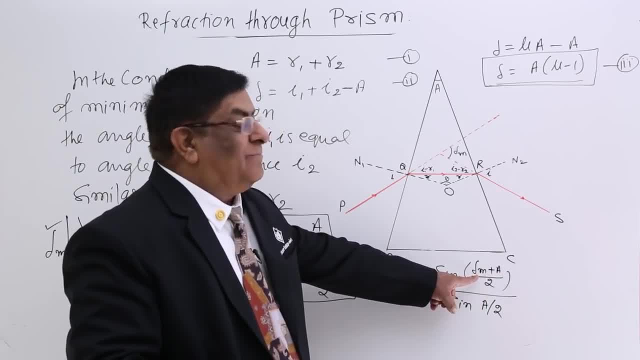 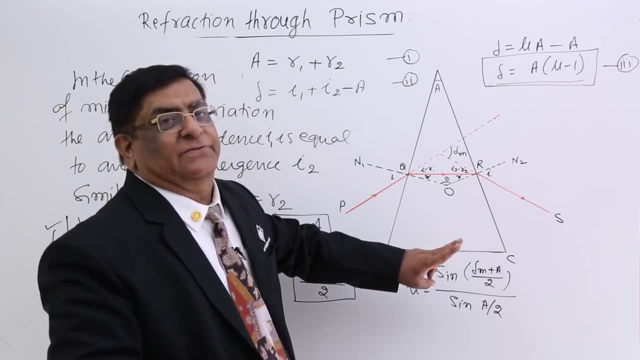 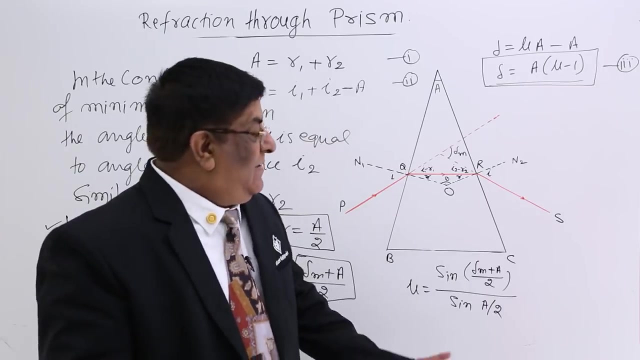 Now here, angle A is known to us delta M. we have found by experiment, So we can find out refractive index of the medium of the press. So this is how we can find out refractive index of the material of the press: by finding: 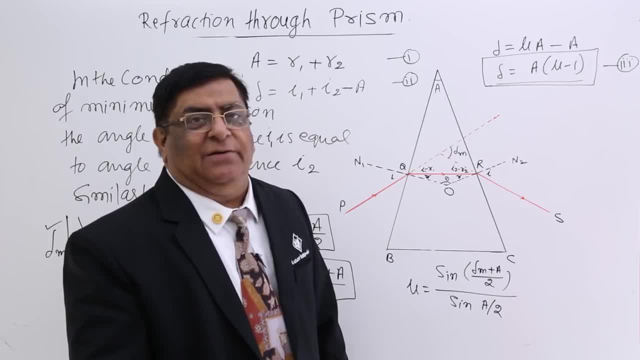 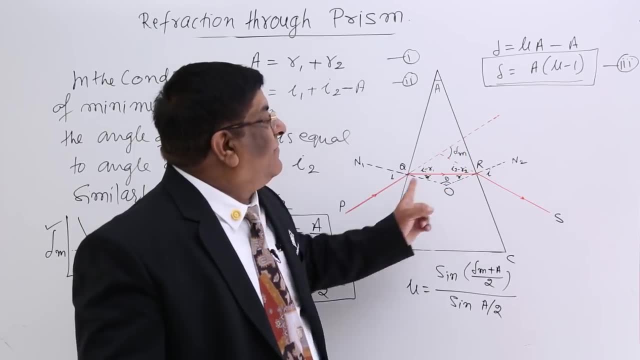 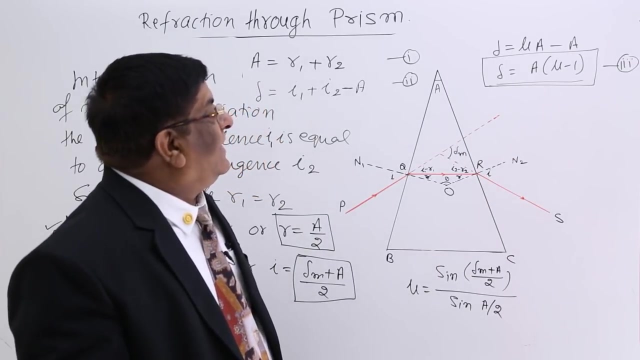 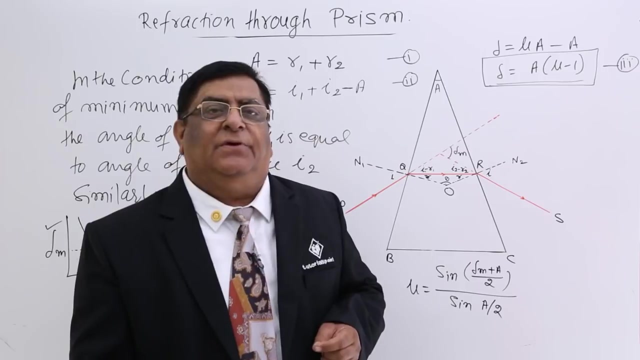 the minimum angle of deviation. We also understand that if we are changing i, there is only one position of i for which delta is minimum. For all other positions, delta will be more than the minimum. Thank You. Now a very important thing here if we want to find out refractive index of a liquid. 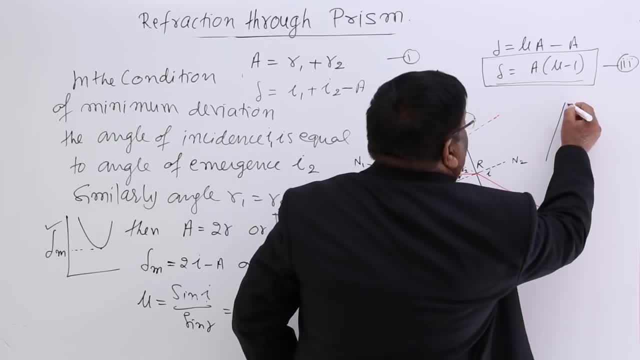 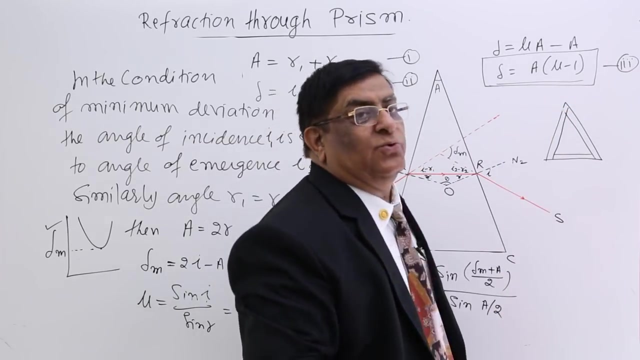 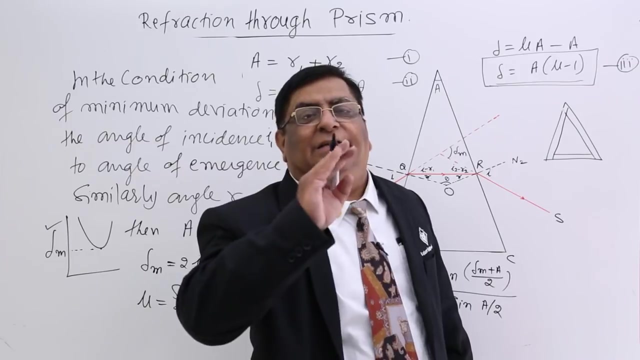 then we make a hollow prism. Hollow prism is made of glass slabs: one slab, two slab, three slabs. Now, these slabs, we have understood they do not do any refraction. That means slab as a whole is not deviating. 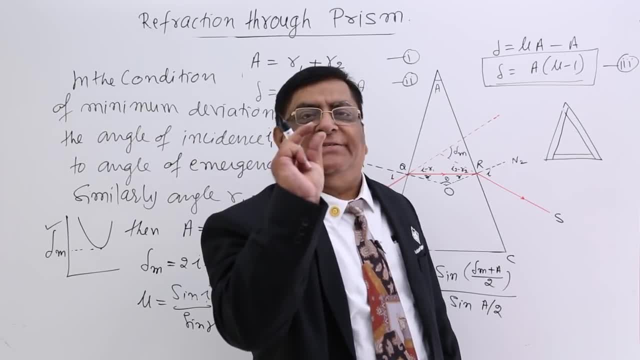 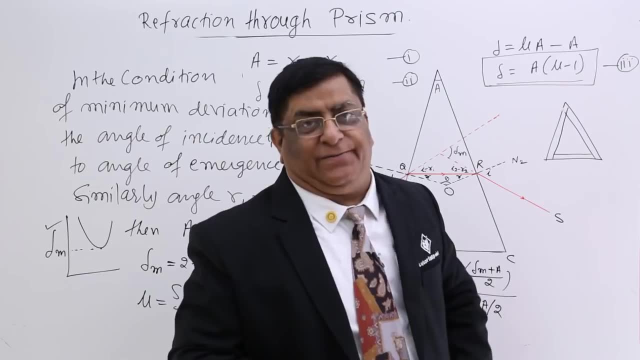 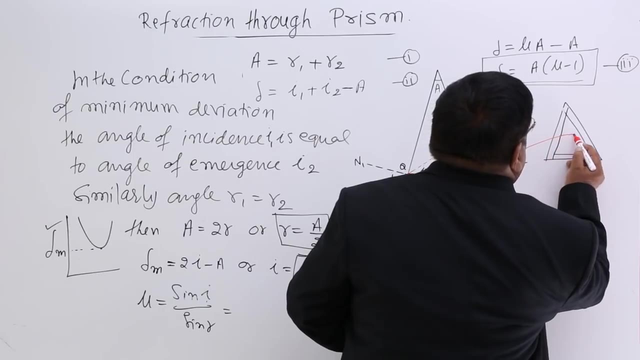 It is only displacing a little, and if thickness is less, then that displacement is negligible, So these glasses will not deviate. Now, if a ray comes from this direction, this, and it goes like this, Then who is responsible for this deviation?